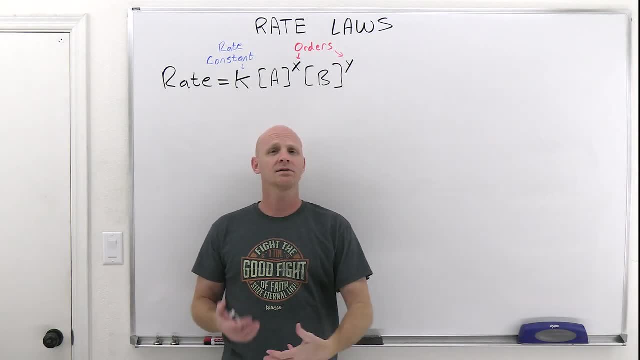 Rate law is going to be the topic of this lesson, and we're going to talk about rate constants, we'll talk about reactant orders and the overall reaction order, but the most important part is we are going to determine the rate law of a reaction based on experimental data, And this is something 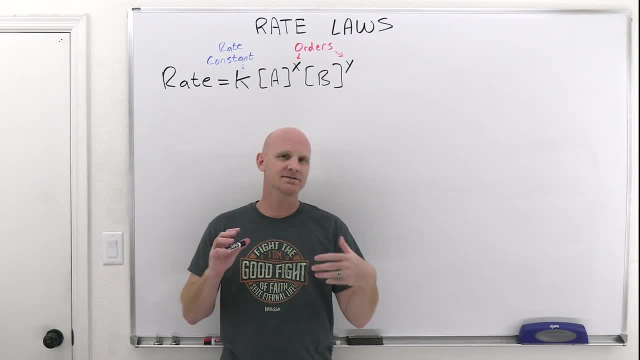 students often struggle with a little bit initially, but we're going to make it simple, I promise. My name is Chad and welcome to Chad's Prep, where my goal is to take the stress out of learning science. Now, in addition to high school and college science prep, we also do DAT, MCAT. 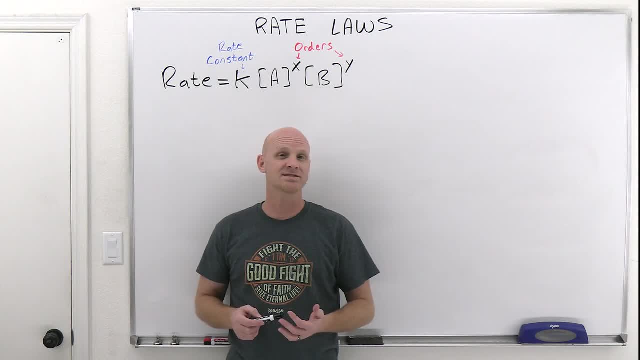 and OAT prep as well. I'll leave some links in the description. Now, this lesson is part of my new general chemistry playlist. I'm releasing several lessons a week throughout the school year, so if you want to be notified every time I post one, subscribe to the channel and click. 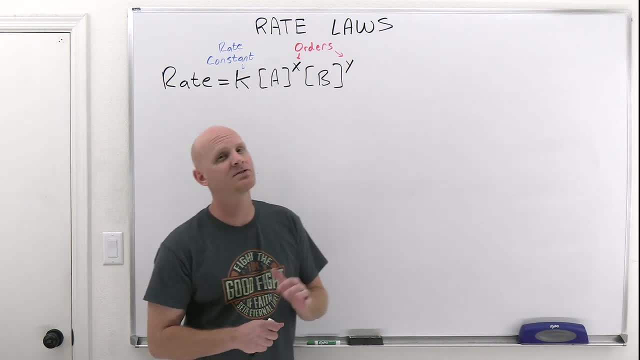 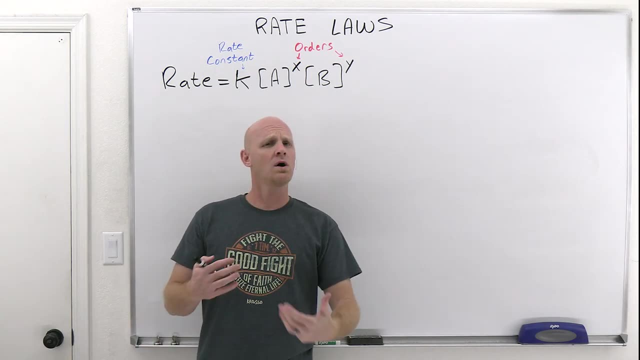 the bell notification. All right, so let's dive in. We've got some vocab to talk about first, and so first let's talk about what a rate law is. And a rate law when you think of, like the laws of nature, like the law of gravity, well, what laws ultimately allow us to do is make. 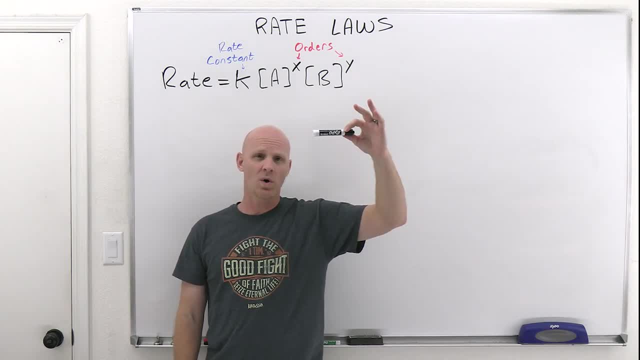 predictions. If I say, if I let go of this marker, what's going to happen? Well, the prediction is that I'm going to be able to make predictions, So I'm going to be able to make predictions. So I'm going to be able to make predictions, So I'm going to be able to make predictions. 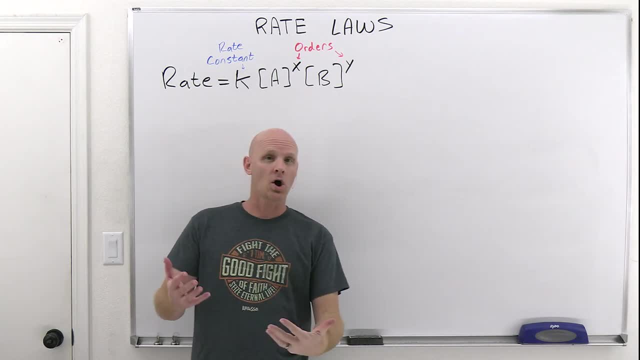 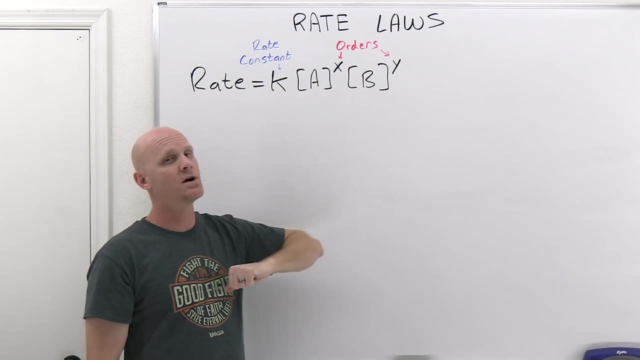 And the prediction is it's going to fall So, and that's based on the law of gravity, And so that's what laws ultimately let us do. is they make? let us make predictions. That's what's going to be true of a rate law as well, And so this is what a typical rate law looks like, And 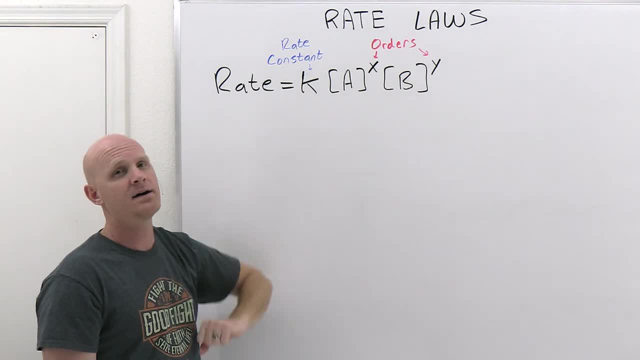 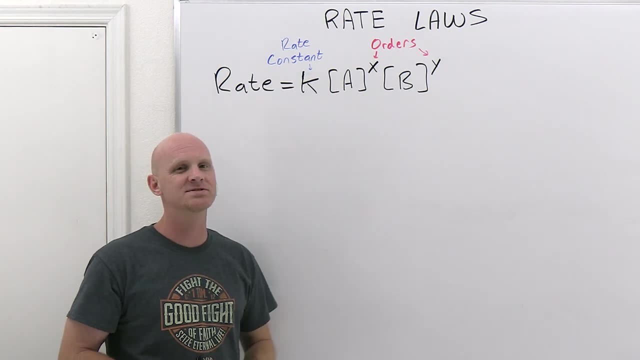 it starts off with a rate constant lowercase K, And it's important to note that it is a lowercase K, not a capital K, because in the next chapter we're going to see something else we use the letter K for, but a capital K as an abbreviation for or a symbol for. So be careful, This is a 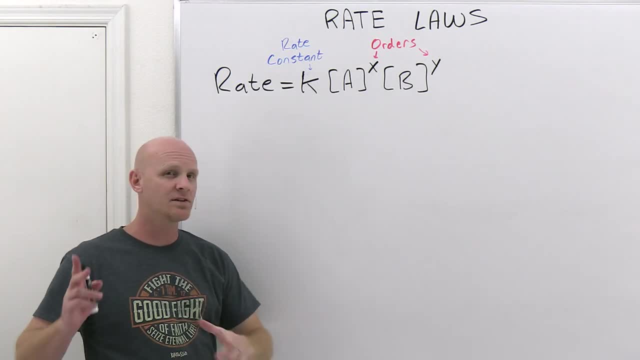 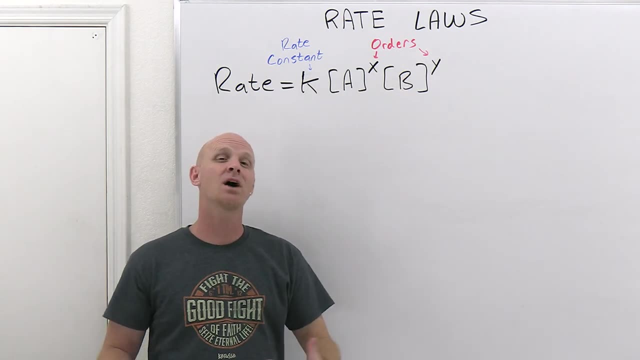 lowercase K. It's a rate constant. It is simply a proportionality constant. We'll talk more about it in a little bit, And then typically reactant concentrations are going to show up. So it's typically just reactants, not products, although that's not exclusive, That's just what's usual. 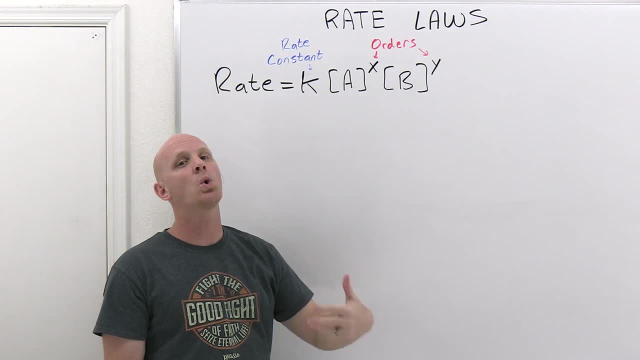 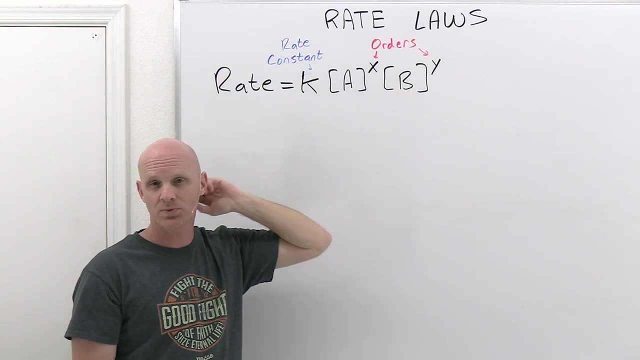 And then you have these exponents right here, And these exponents are called the orders, And so X would be called the order with respect to reactant A, Y would be called the order with respect to reactant B, And then there's also it's called the overall reaction order, which is the sum of 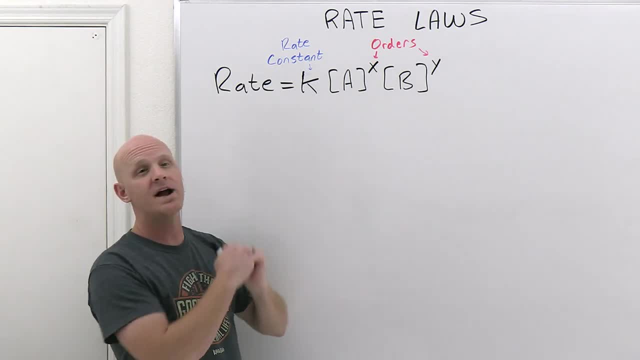 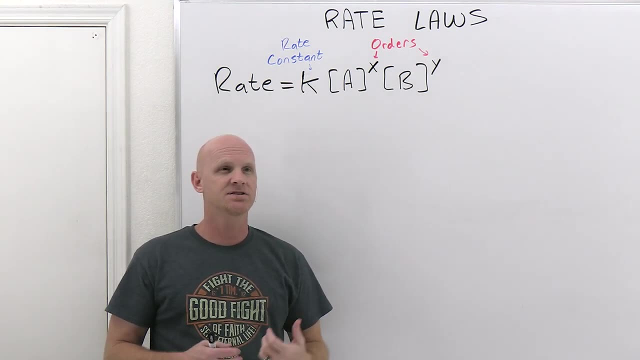 all the individual reactant orders, And so in this case, the overall reaction order would be X plus Y. Now, these orders are very commonly integers, and they're sometimes related to how many of that particular molecule is involved in what we're going to call the slow step in a reaction. 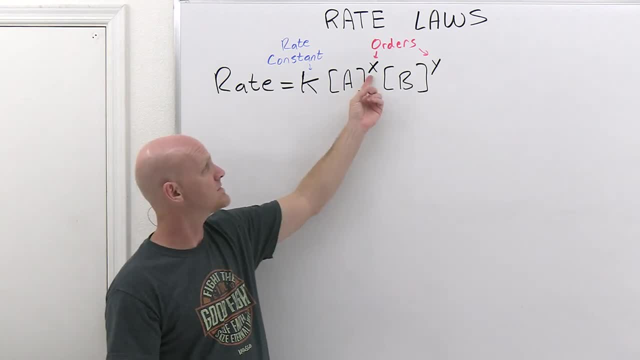 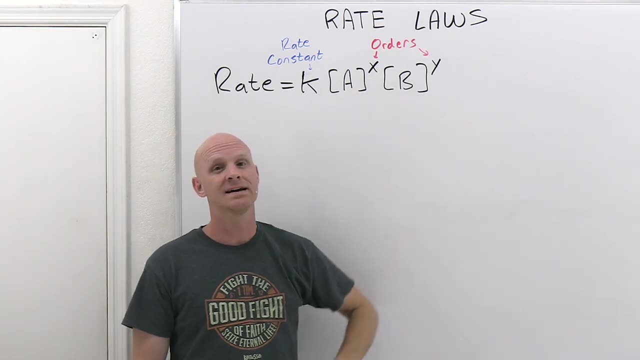 not necessarily in the overall reaction. And so it turns out. you know, sometimes these are going to match up with the coefficients in reaction and sometimes they're not. So you can't just look at the coefficients in reaction and be like, oh, those are the orders. It sometimes just happens. 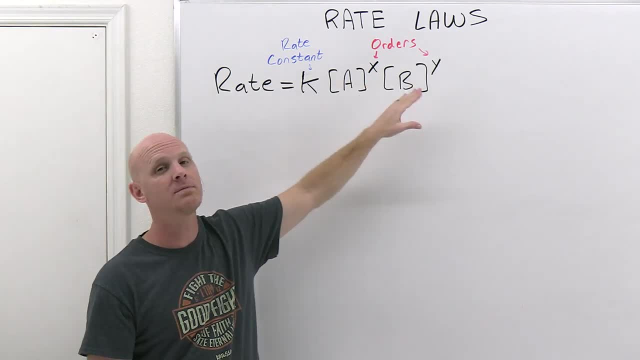 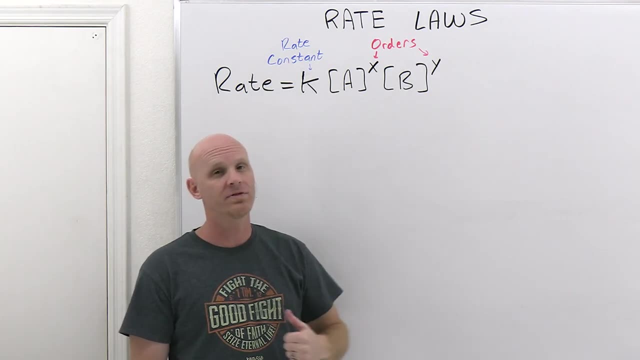 that way, but it's not necessarily going to be the case. So it turns out you're going to have to determine these and get the rest of the rate law here from experimental data. You can't necessarily just tell by looking at a reaction what those are going to be. All right, So again, these are very 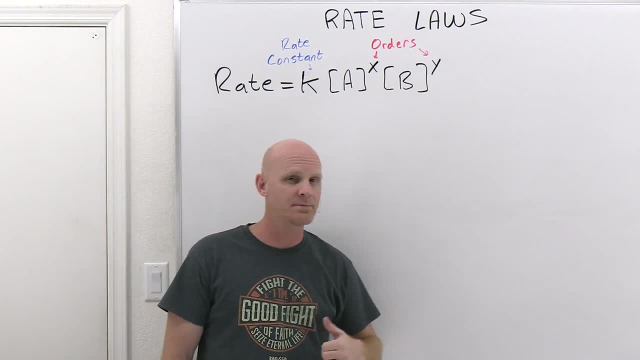 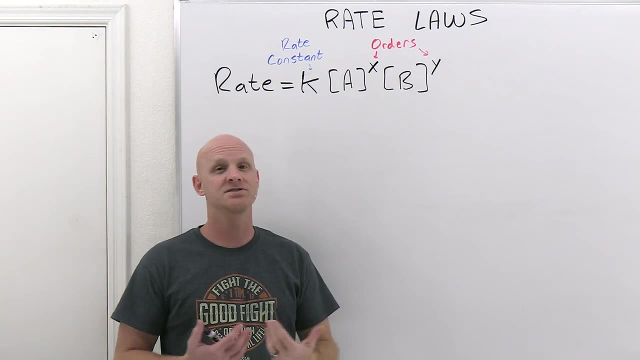 often integers, and 0,, 1, and 2 are the most common by far. However, in principle, like with you know, if you're going to use some actual kinetics, experimental data, you know these can come out to fractions or decimals and things of this sort. However, you're going to find in your 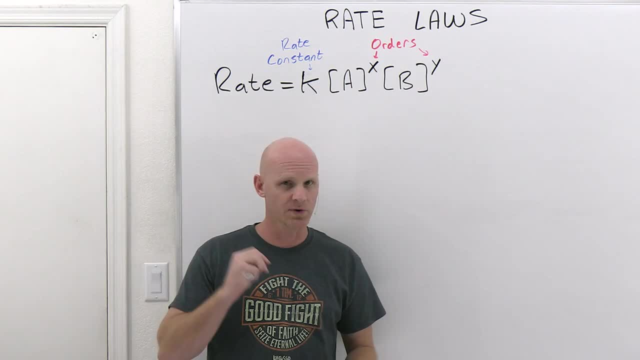 most commonly, you're either going to see 0,, 1, or 2.. However, if I make the statement that reactant orders are always integers, you should know that that is false. So, however, almost exclusively the ones you're going to see in this chapter are going to be integers, which is why 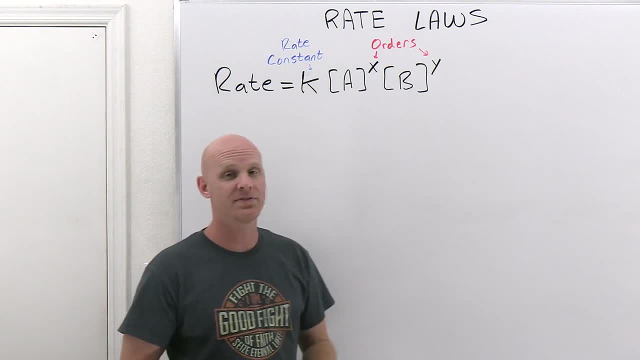 that makes that statement a tricky, true-false evaluation. So, but they don't have to be integers, just most commonly, that's what we're going to see, And again, they're most commonly 0,, 1, or 2.. 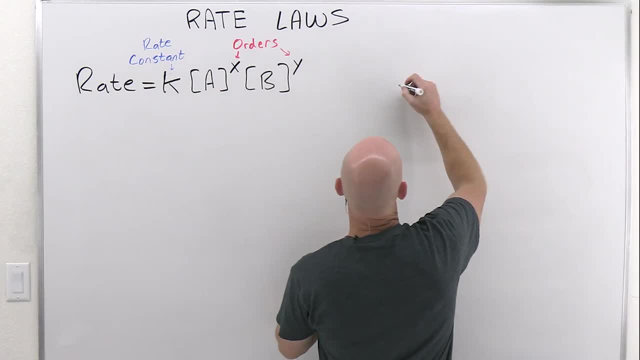 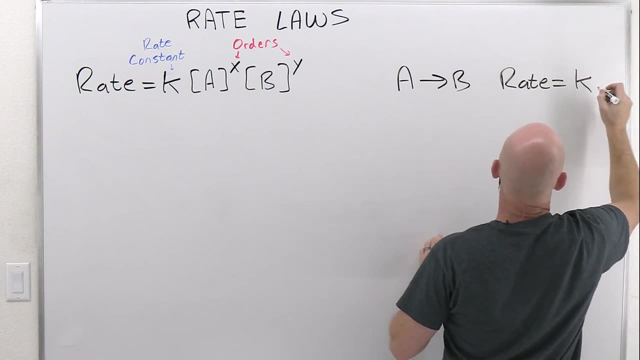 So we're going to take a look at a few reactions here. And so let's say I've got a reaction of A going to B and I tell you that the rate equals K times A to the 0 power. Now I'm telling you: 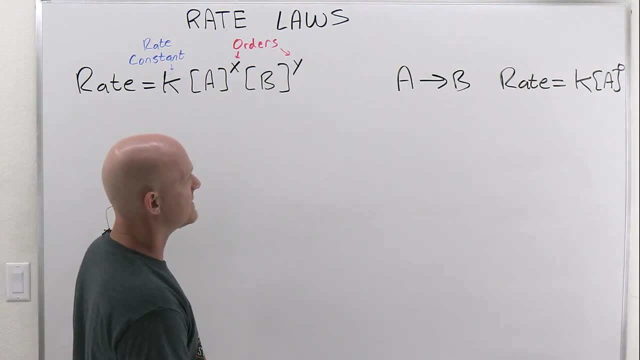 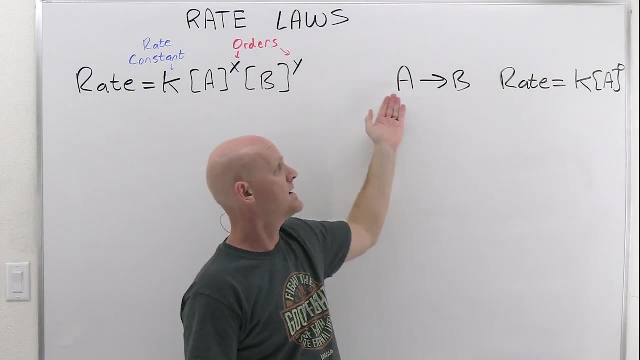 it's K times A to the 0 power. That's telling you there that the reactant order with respect to A is 0.. So, however, with only one reactant here- so notice that's the only reactant showing up in the rate law- then the overall reaction order is 0 as well, And that's what I really want to focus. 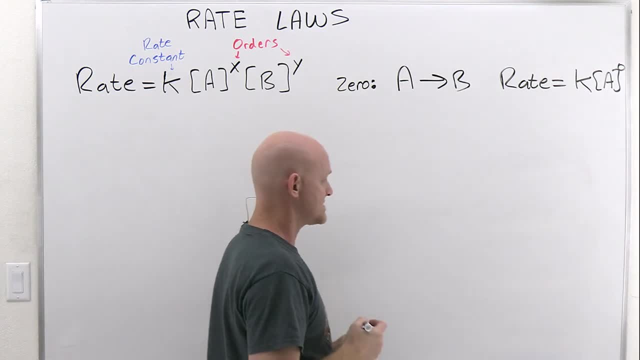 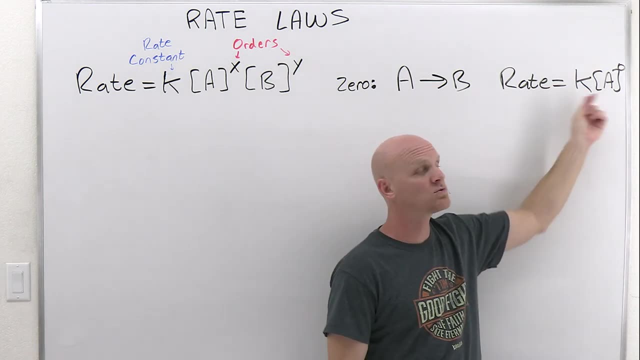 on. here is something that is 0 order, And so, in this case, also notice that anything to the 0 power equals 1.. And anything times 1, notice K times 1.. And again, it doesn't matter what concentration. 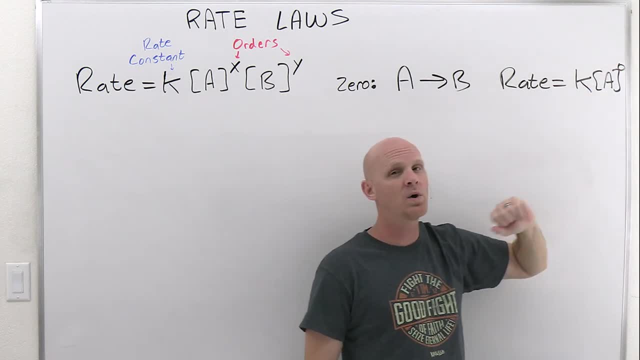 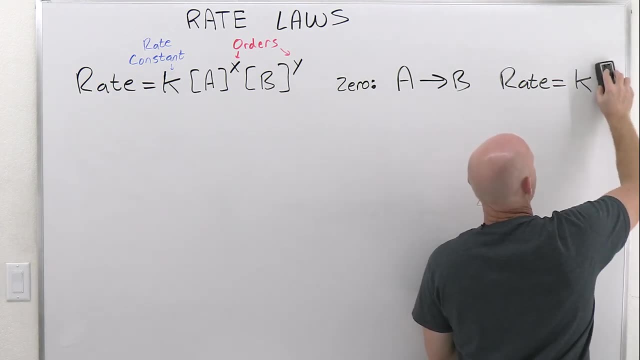 of A- you plug in anything you plug in there to the 0 power equals 1, and K times 1 is just equal to K, And so oftentimes you'll just see this written without any reactant concentration listed there at all, because it doesn't matter And that is the hallmark of a 0 order reactant, is that? 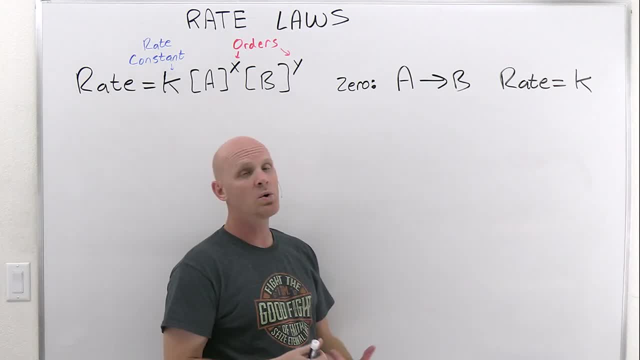 anything to the 0 power equals 1.. And so in this case, also notice that anything to the 0 power, its concentration, doesn't affect the rate at all. You want to put in 1 molar A, the rate equals K. 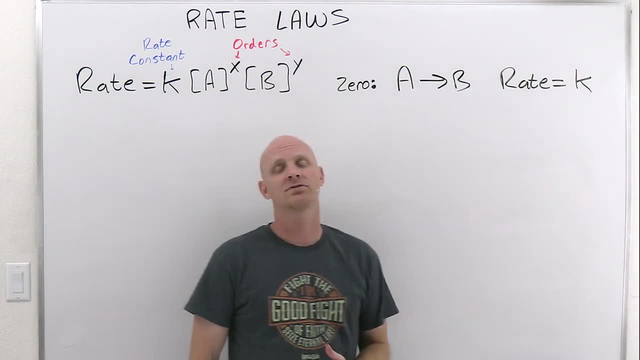 You want to put in 10 molar A, the rate equals K And so the rate is not affected by a 0 order reactant. All right, next we're going to take a look at a first order reactant. So, and for this one we're going to take a look at a fictitious reaction M. 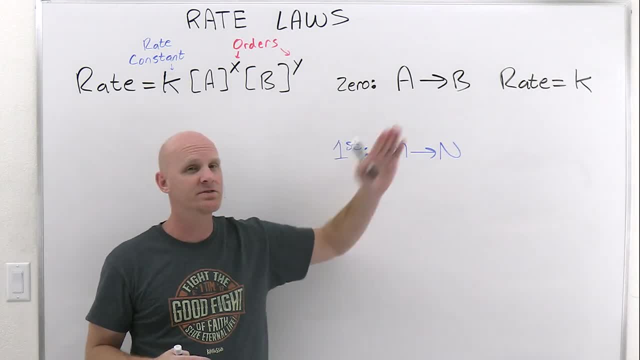 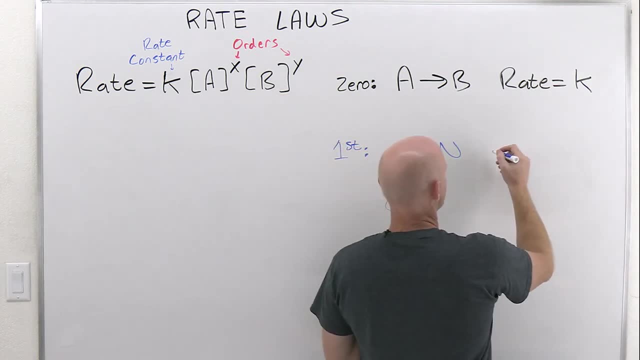 going to N. I prefer to actually just do A going to B every time, but I really want to distinguish this and I don't want this to get confusing. So, but M going to N here, and so again, M is typically going to be what shows up in the rate law, And so here, 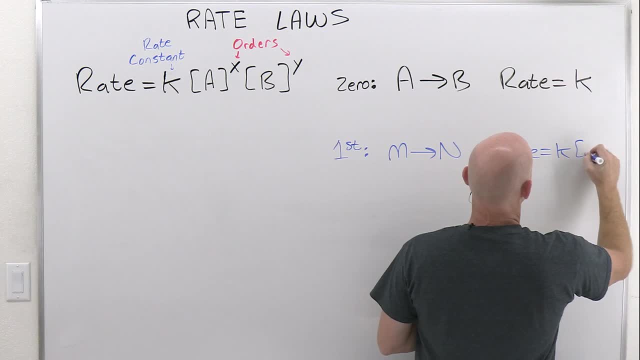 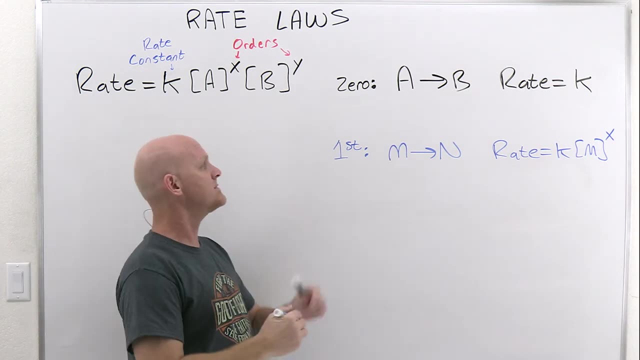 we're going to have rate equals K times the concentration of M to some power here, And that power, again, you know, is often integers, doesn't have to be. But if I'm telling you it's a first order reactants or reaction in this case, then I'm telling you that that right there is. 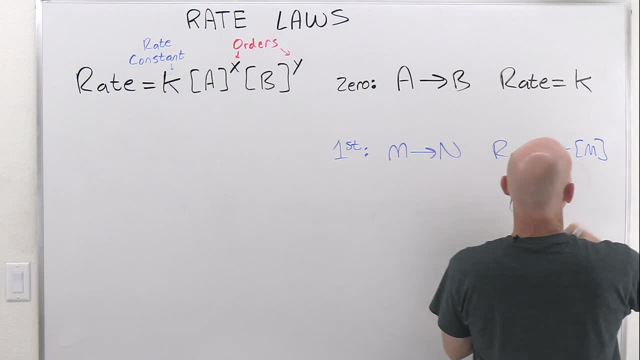 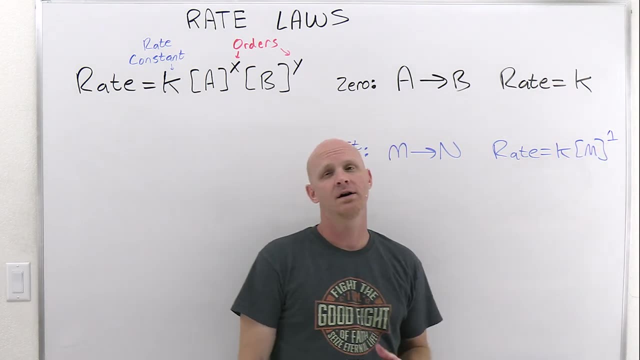 going to be a 1.. And so we'll substitute a 1 in there. That's what makes it a first order reaction here with only one reactant. That one reactant is going to be first order. But notice anything to the one power is itself. So, like three to the one, power is three, Five to. 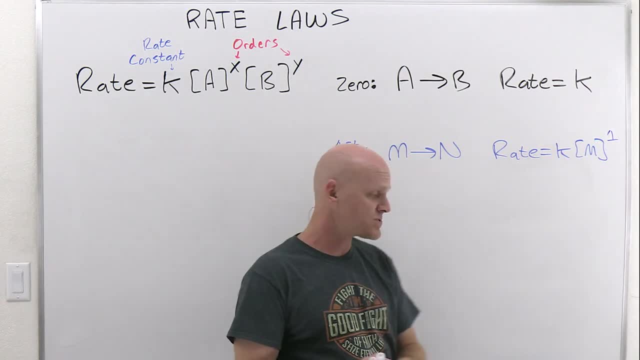 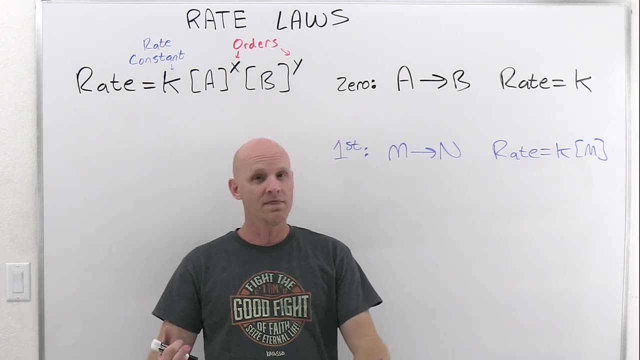 the one power is five. Well, the concentration of M to the one power is just the concentration of M, And so you often see that completely omitted So, and it's just implied that there's an exponent of one there, And so this is what typically a first order reaction looks like. 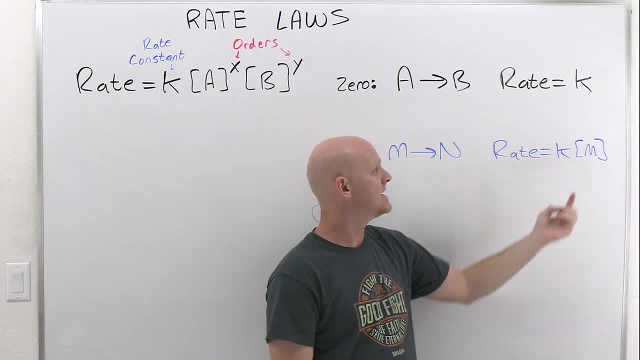 And what you see here is that the rate is proportional to the concentration of M. If you double the concentration of M, it doubles the rate. Notice, if I have one molar M, well, one times K is K. And then if I do a second trial of this, but I use twice as much, twice. 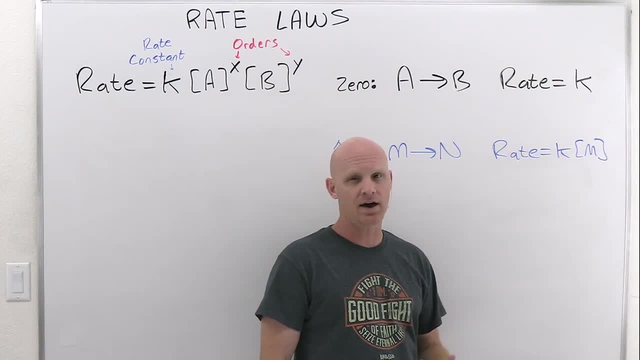 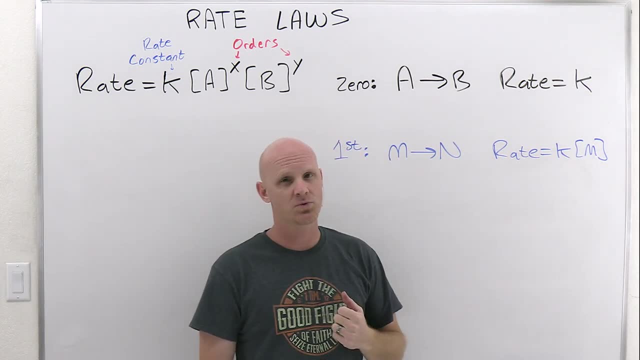 the concentration of M. So two molar M, well, two times K is two K, and two K is double the value of one K. And so, doubling the concentration of M, doubled the rate of the reaction. And so this is the hallmark of a first order reactant, where, you know, again, in contrast to the 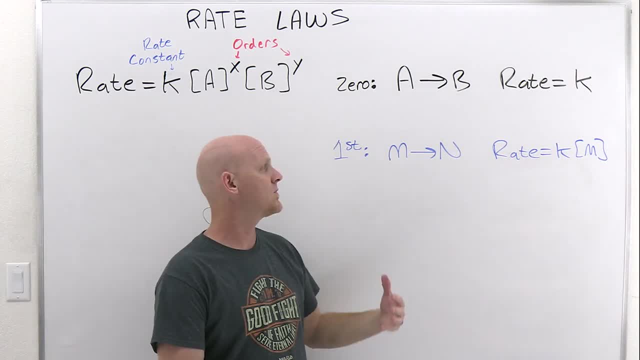 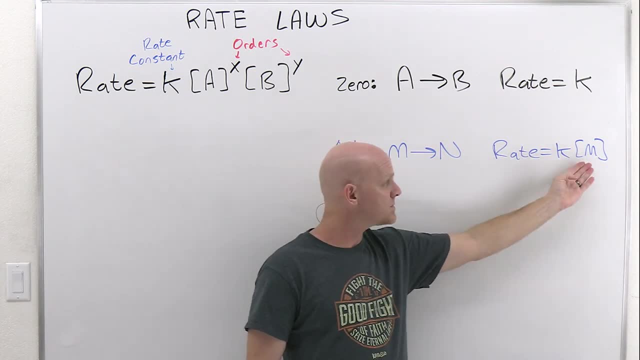 zero, where the concentration of that reactant doesn't affect the rate at all. So here with a first order: the rate of the reaction is proportional to that concentration. You double the concentration of M, The rate doubles. You triple the concentration of M, The rate triples. You increase the concentration. 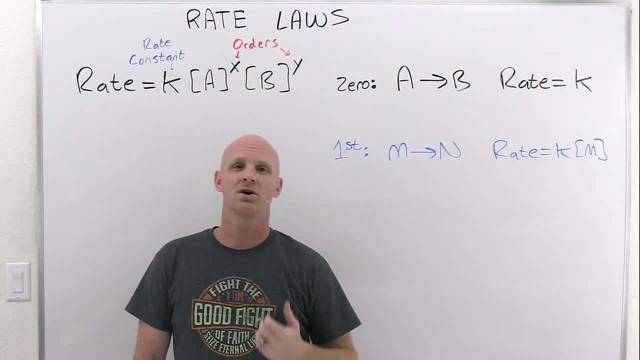 of M by a factor of 10. The rate's going to go up by a factor of 10.. So, and that is the hallmark, again, of first order, And so, when you're looking at experimental data, if you look at how you know, what we typically are going to do is run two independent trials. 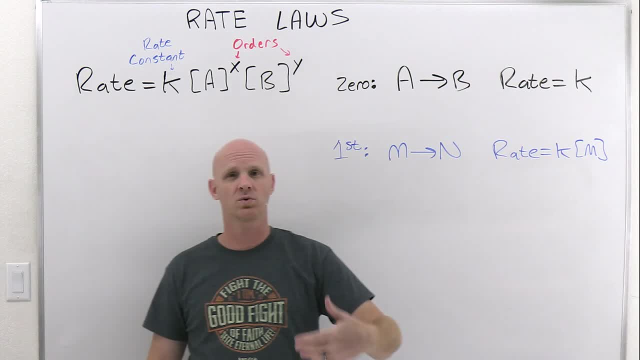 where we say, vary the concentration of M, We might double it or triple it or quadruple it or cut it in half, or we're just going to have two different concentrations And then we're going to see what happens with the rate. We'd actually measure the rate of 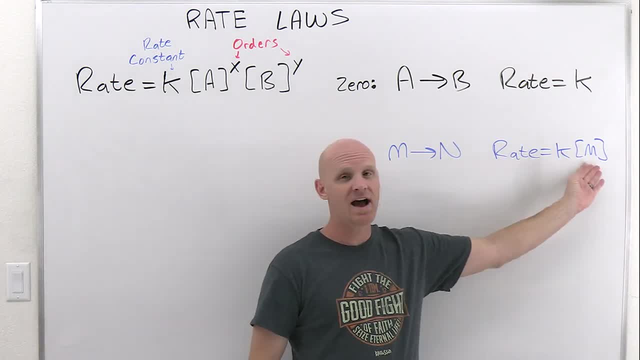 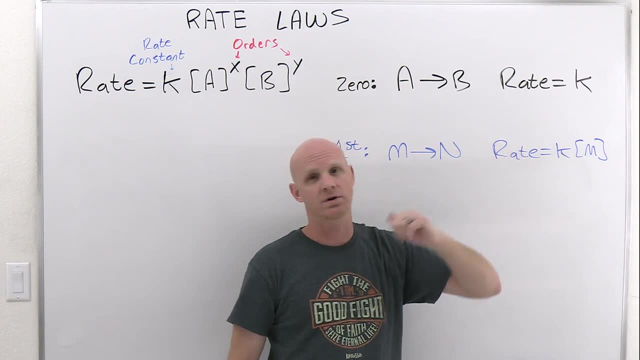 the reaction and see what happens. And if the rate does exactly what that concentration does, that's the hallmark of a first order reactant. So again, if you double that concentration of M and the rate doubles first order, if you triple it and the rate triples first, 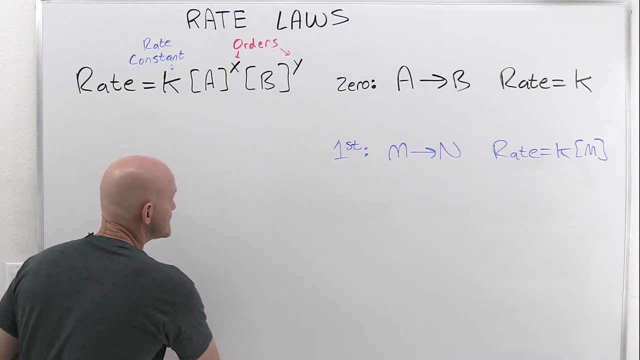 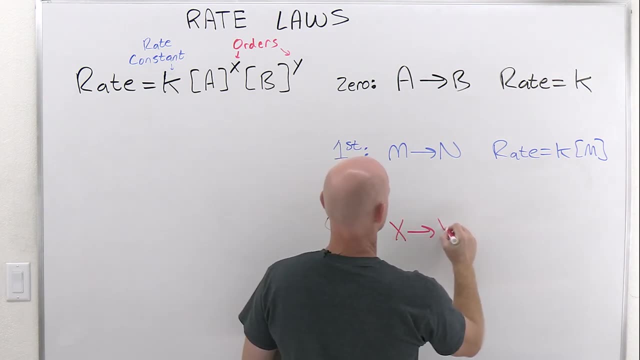 order. All right. Last but not least, we'll take a look at second order reactions. So in this case, I'm going to do X going to Y, And so X being the reactants, typically what's going to show up in the rate law. So, and in this case, what makes it second order is it's going: 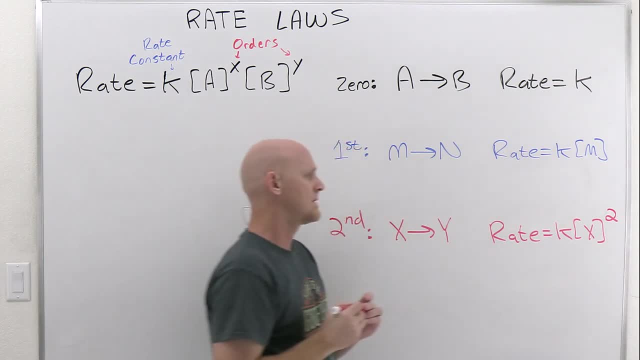 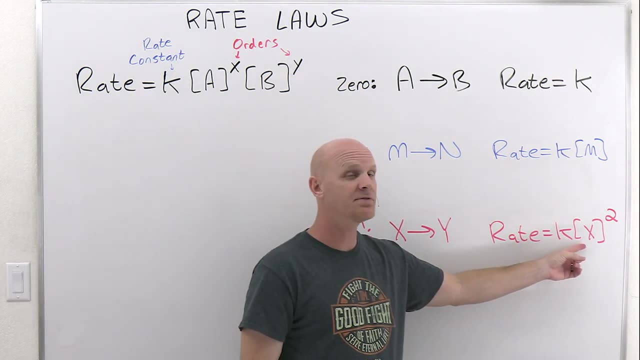 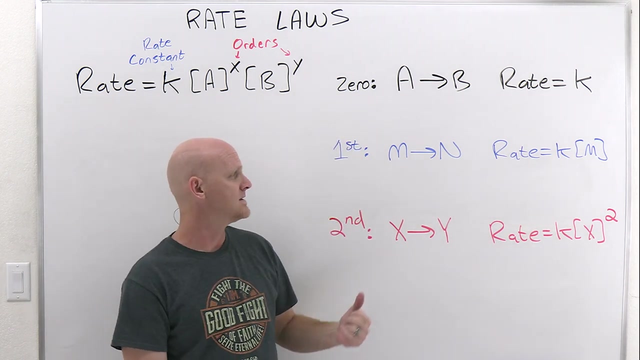 to have an exponent of M, And so, in this case, what this ultimately means is that now the rate is not proportional to the concentration of X. now it's proportional to the concentration of X squared, And so this means that the reactant X has an even bigger impact than the reactant M. 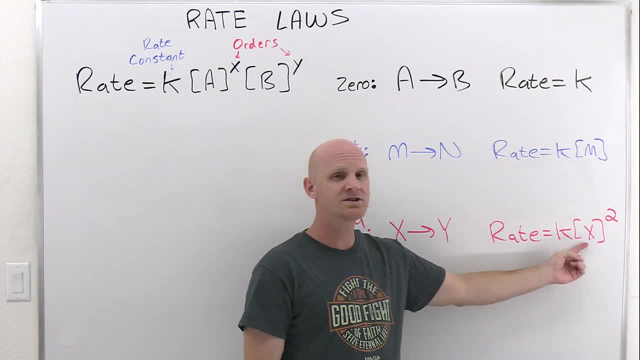 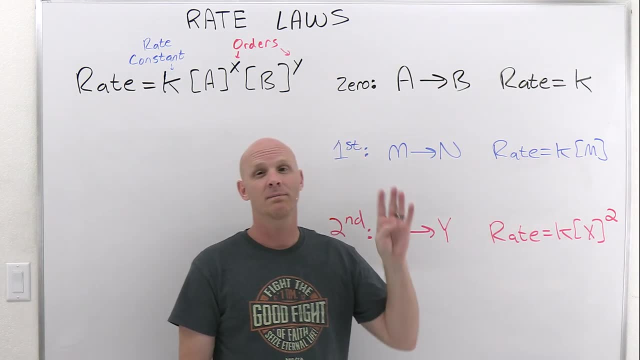 here had on the rate. So now, if you double the concentration of X, well, doubling squared is four, And so if you double the concentration of X, it's actually going to increase the rate by a factor of four. And so whatever you do to the concentration, the same thing is going to happen to the rate. 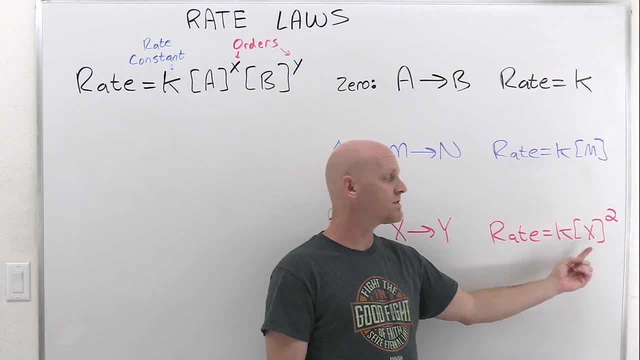 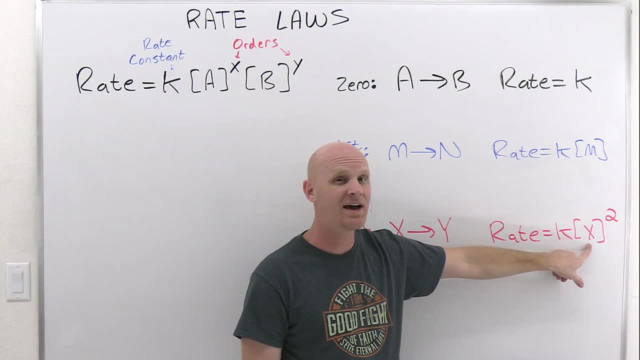 but squared. And so if you triple the concentration of X, well, three squared is nine. That means the rate's going to go up by a factor of nine. If you increase the concentration of X by a factor of 10, well then the rate's going. 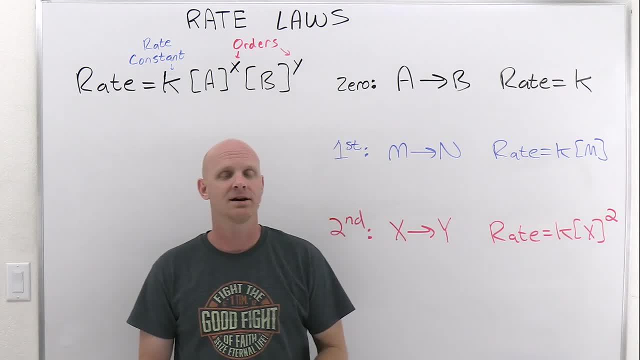 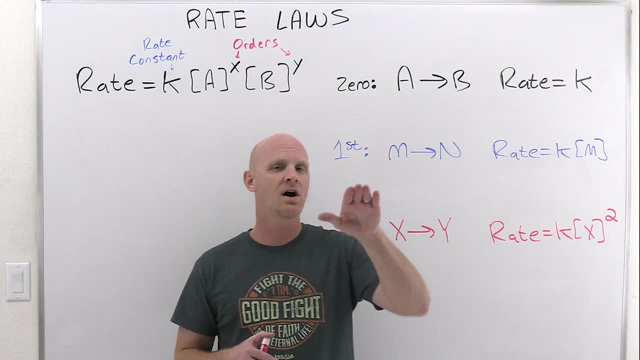 to go up by a factor of 10 squared, or a hundred in that case. And so again, when we're going back and looking at some experimental data, when we look at two different trials and we say, oh, look at those two trials. the concentration of 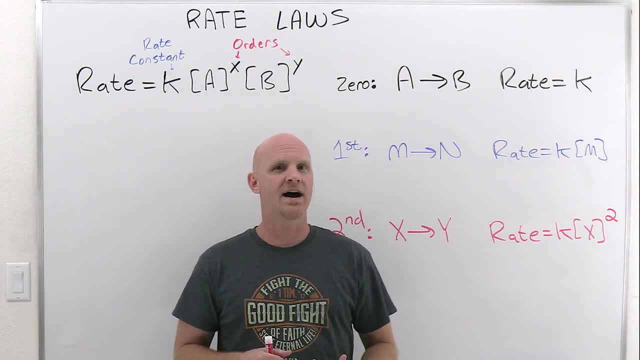 whatever tripled there, And then the rate went up by a factor of 10.. The rate went up by a factor of nine. well, tripled squared is nine, And that's how we'd determine if it's a second order reactant. 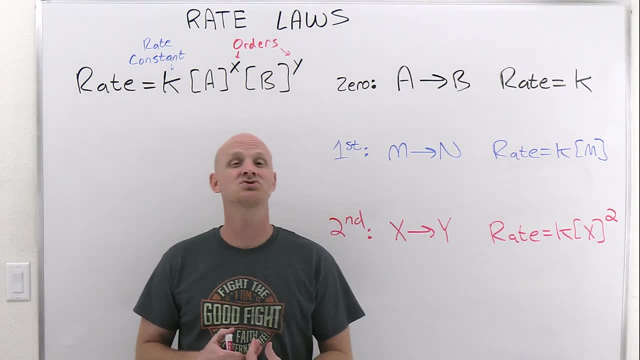 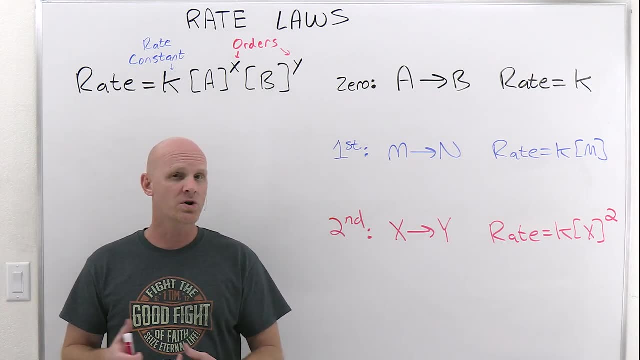 Now, in principle you can also have, say, a third order reactant. They're super rare, super uncommon and you're not likely to see them, But in principle it would work the same way. If you had a third order reactant, well then you know, doubling its concentration would. 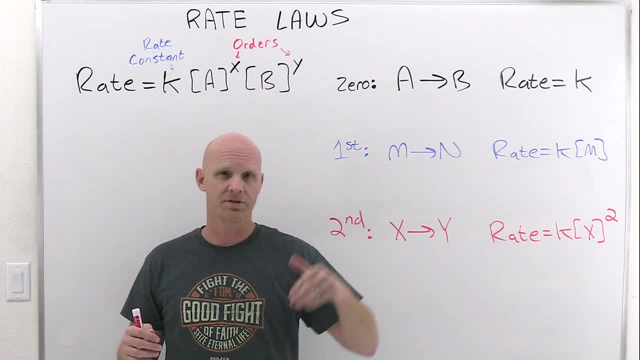 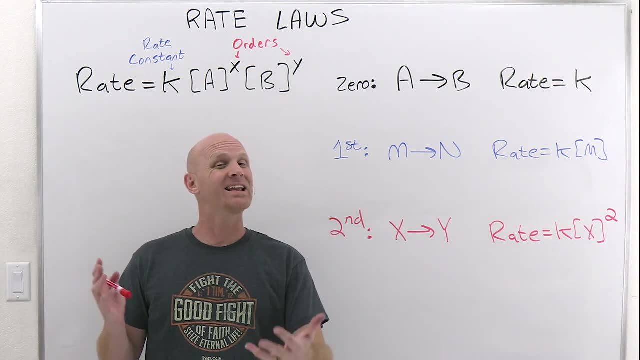 cause the rate to go up by double to the third power and double to the third power. two times two times two is eight times, uh, eight fold increase in the rate in that case. Now again, you're not lucky, You're likely to see that, but in principle it works, in kind of the same sense of what 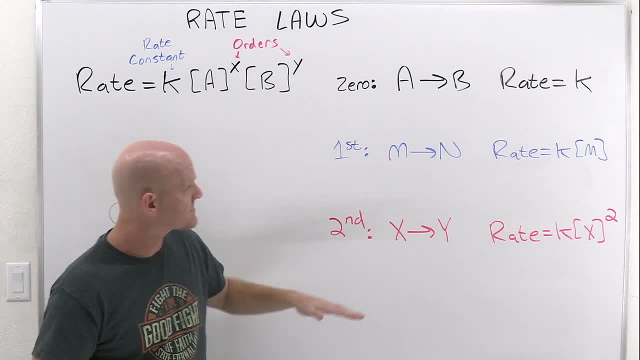 we're doing here as well. Okay, So these are the three most common orders, but once again, fractions are possible, decimals are possible, But again, in this chapter, this is probably all you're likely to see If you end up doing any kind of kinetics experiment in your lab. all bets are off, though. 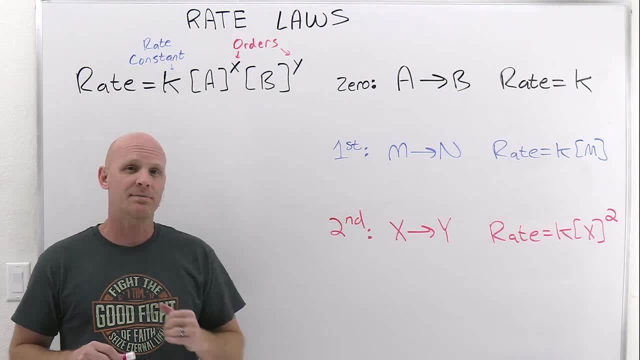 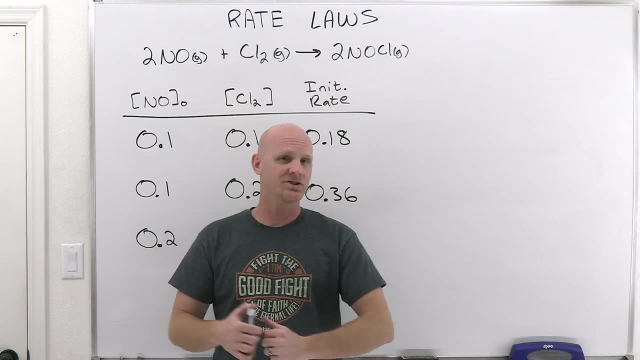 Just an FYI. All right, let's take a look at examining some experimental data. All right, So before we look at some experimental data here to determine a rate law, just want to kind of give an analysis. So let's say that I've got a vehicle and I walk out and I turn the key on my vehicle. 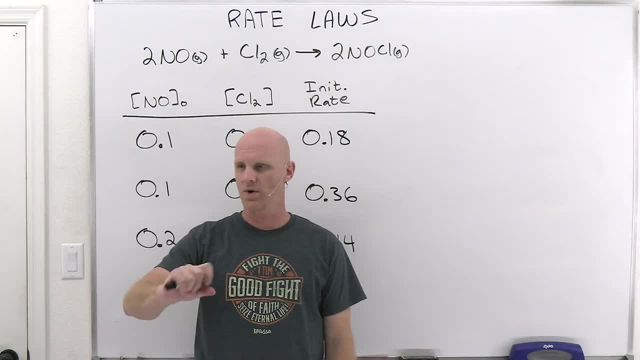 and this actually happened to me this week, and nothing happens. No engine turnover, not make doesn't make a sound. So in the question is: well, what could be the problem? So, and don't say out of gas, if you see, you know, if I was out of gas the engine would. 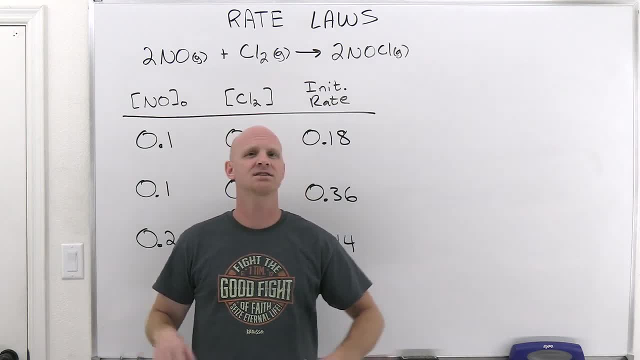 still try to turn over, just wouldn't start, So. but here's nothing, doesn't make a sound. So what could be the problem? Well, I could have a dead battery. that could definitely be the issue, or other common option would be: I have a dead starter. 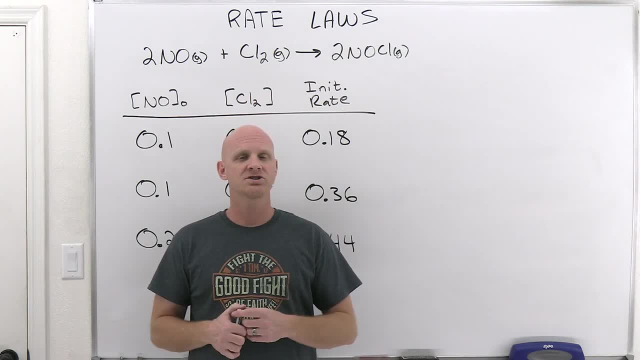 So, and those are probably the two most likely scenario, And so the question is: well, which one is the problem? So? and let's say, I can't afford to take this to a mechanic and I need to fix it myself, But I don't know how to diagnose which one it is. 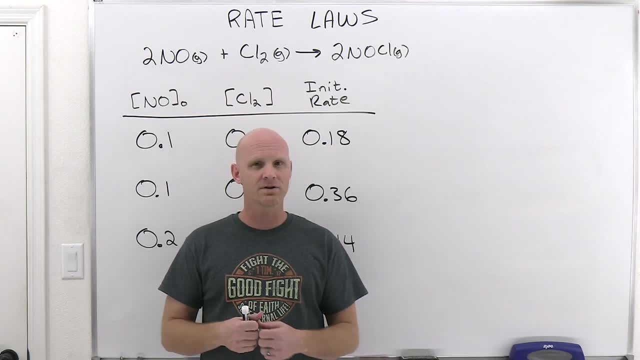 I don't have a battery tester. I don't know how to test a starter, you know with voltmeter or anything like this. So how do I figure this out and how do I replace this at the most economical way? Well, what you do is you go to your local auto parts store and you buy a brand new starter. 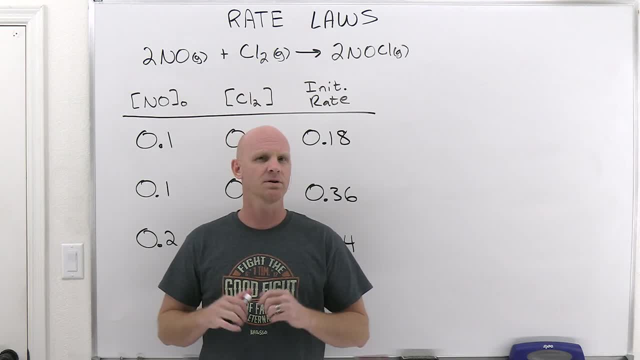 for your vehicle and a brand new battery for your vehicle and you're replacing both. Okay, And that's the most cost effective way? Okay, that's not the most cost effective way, because why replace both of them if only one of them is the problem? 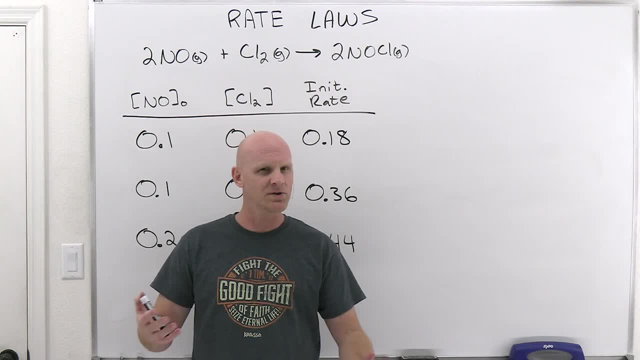 So, again, you can't afford to take it to mechanic, so you can't afford just to replace parts you don't need to replace, And so what you're going to do here is you're actually still going to get again, buy both of them brand new and you hold on to that receipt. And so what you're going to do is you're just going to replace one at a time, Because if you replace both and then your truck starts, well, then you still don't know which one was the problem. But let's say you just replace the battery. 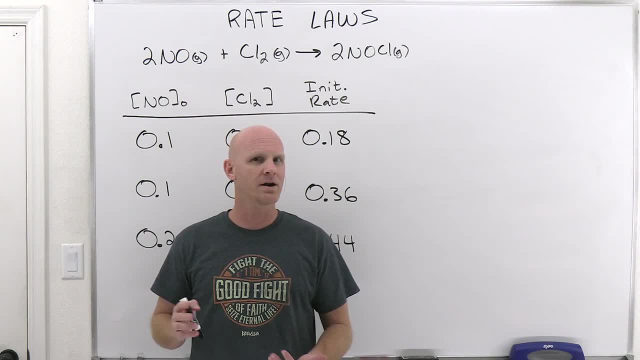 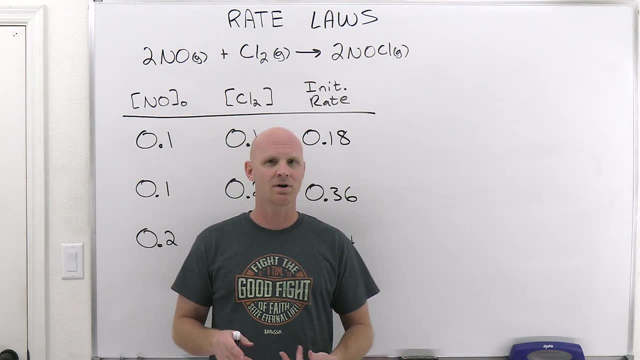 And the truck starts, well then you know the battery was the problem. But let's say you replace the battery and the truck doesn't start. well then you know the battery wasn't the problem, And in that case you'd put the old battery back in and then you'd swap out the starter. 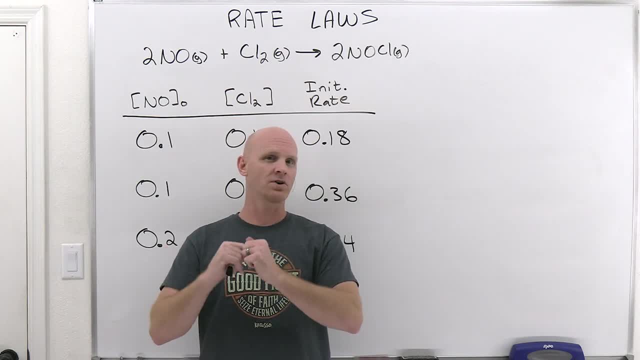 And if replacing only the starter and the truck starts, well, then you know the starter was the problem, And the idea is that you want to only change out one of the variables here- battery or starter- at a time, so you'd know what impact it actually has. 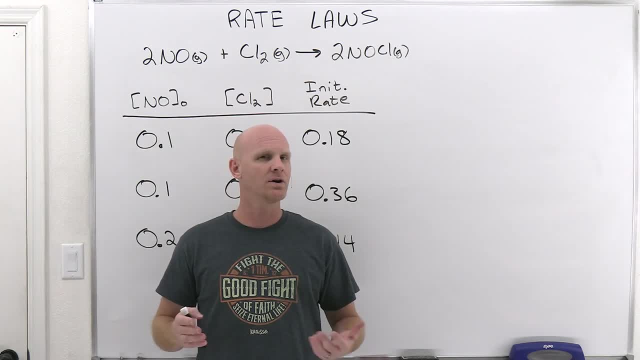 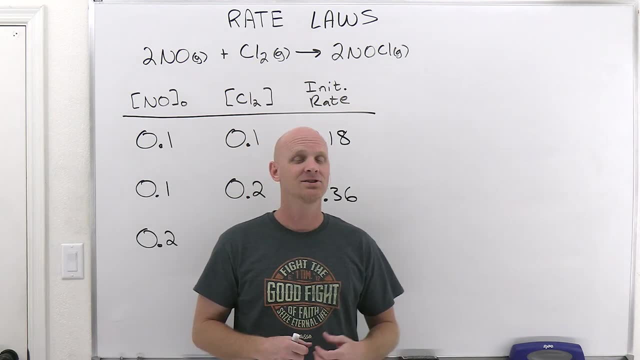 Okay, And if you replace both out at the same time? if it fixes the problem, that's great, but I just don't know which one was really the one that fixed it, and I don't know which one. to return back to the auto parts store to get my money back. 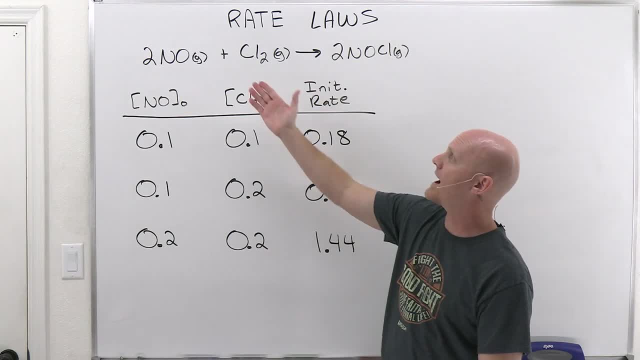 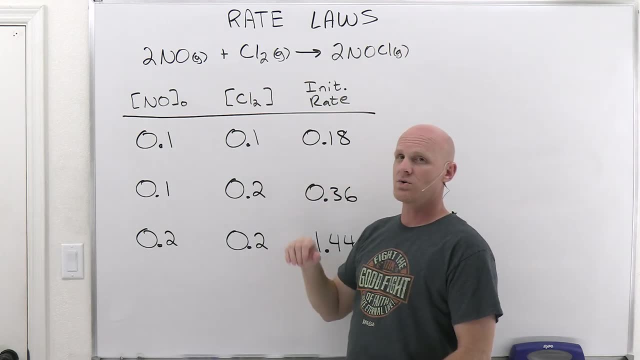 So that's kind of the idea here. So what we're going to do is we're going to look at a reaction here between NO and CL2 to make NO-CL, And we're going to look at three different trials we ran. So what we're going to do is we're going to do three independent trials. 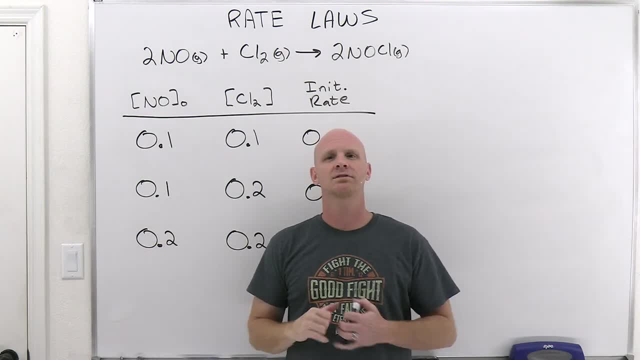 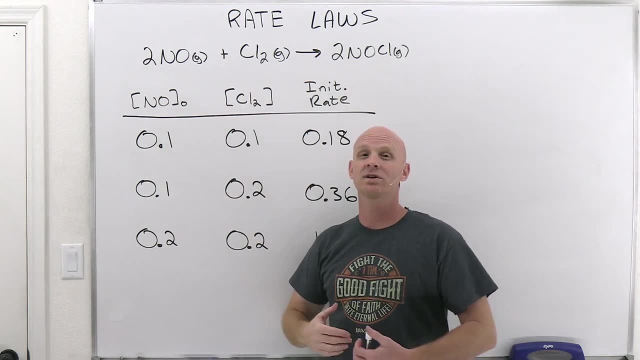 We got three different test tubes or three different beakers or something like that, And we're going to put in different concentrations of CO2.. We're going to put in different concentrations of the reactants NO and CL2.. And by differing those reactants we're going to see then, well, what impact does that have? 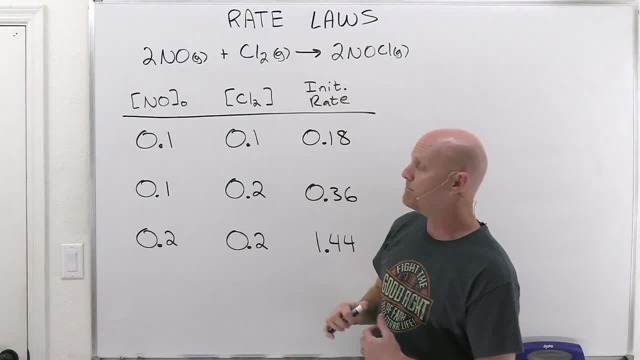 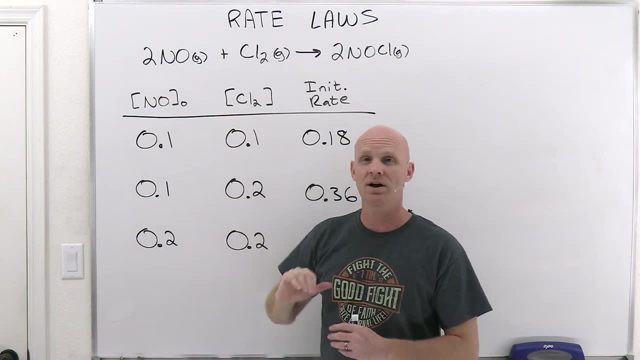 on the rate. We'll measure the rate going on in each one of these beakers, test tubes, whatever, And so, in this case, what we want to do, then, is compare two trials, and in the second trial, we just want to change just one of the reactants, only one. 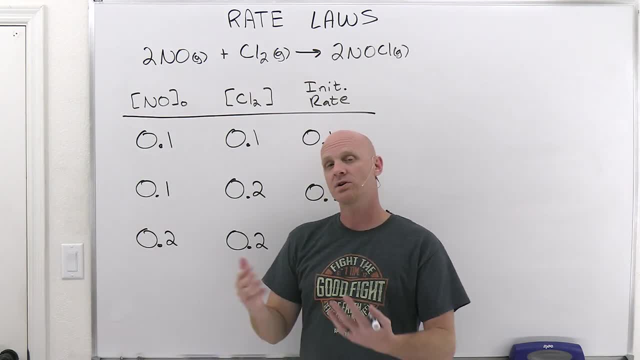 If we change them both and the rate changes. I don't know which one to attribute the change to. Was it because we changed the NO? Was it because we changed the CL2? I don't know. Was it both? It was both. 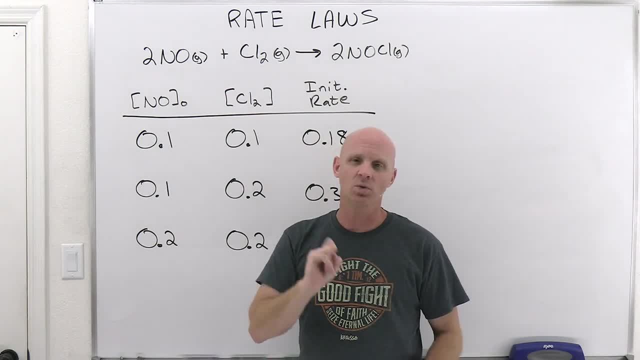 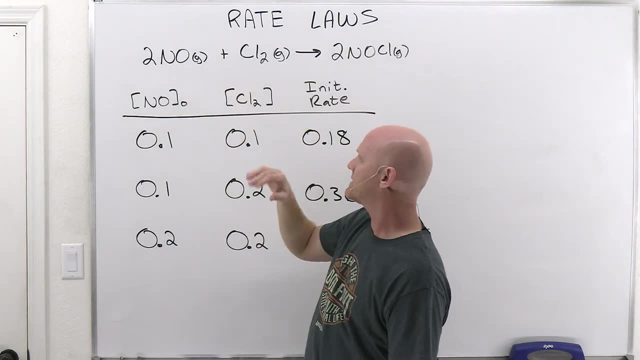 But if I change only one of them and the rate changes, I know which one is responsible for that change in the rate, the only one that I changed. And so in this case, like, if we take a look at, NO, if I want to pick two trials either, 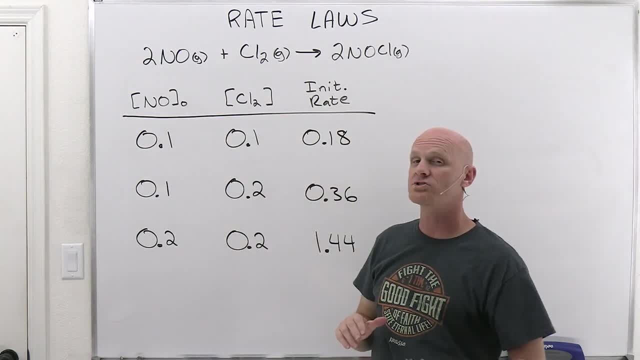 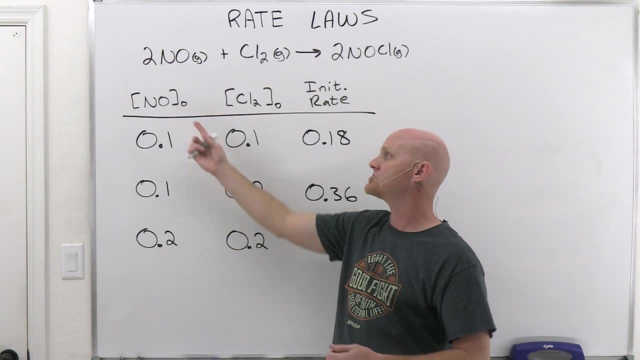 the first trial, the second trial and the third trial, two out of those three and I want out of the two initial concentrations. so in that little zero there means at times zero, it just means initial. so initial NO concentration. initial CL2 concentration. 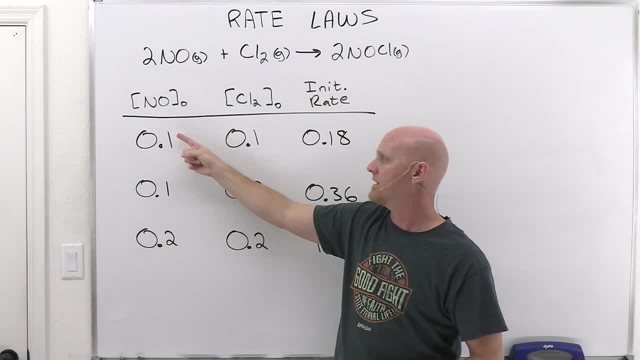 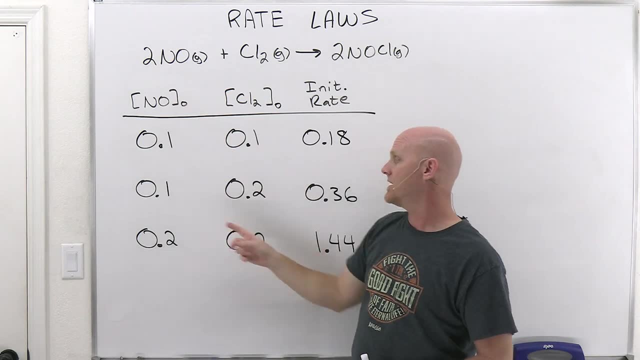 And if I want to pick two trials where only this is different And notice the first two, that's not going to work. Now the second and the third looks like it'll work, but I got to make sure that it's the only one changing. 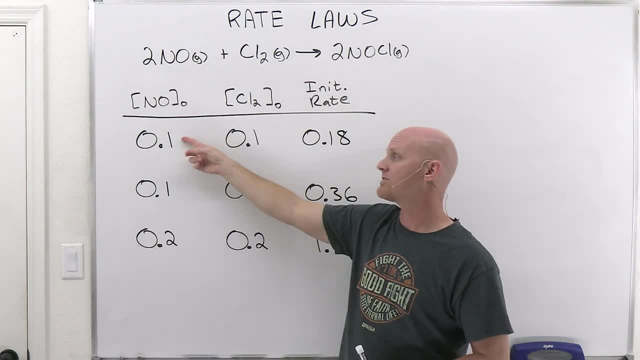 And that is totally the case. Now notice these aren't in any particular order. I could have compared the first to the third, but that would have been a problem. If I compare the first trial to the third trial, the NO changes, and that's good, because 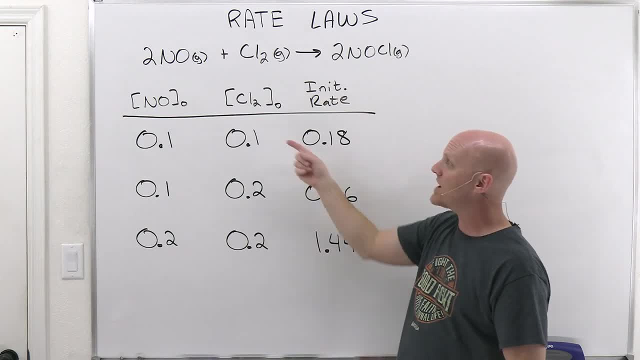 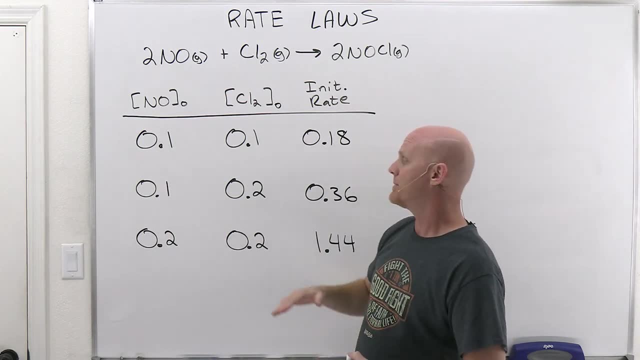 I can evaluate whether that change has an effect. The problem is it's not the only change, because the CL2 concentration was changed as well. So that would not be a comparison that's going to benefit us at this point. but comparing trial two to trial two, 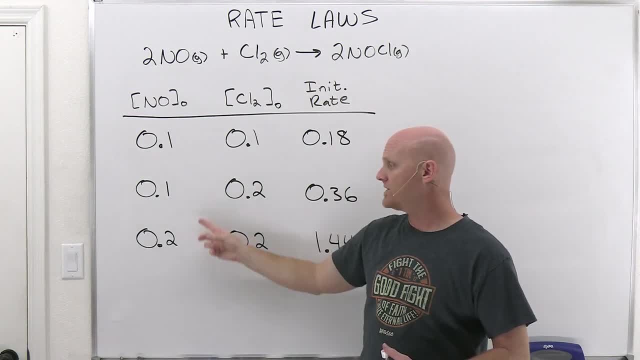 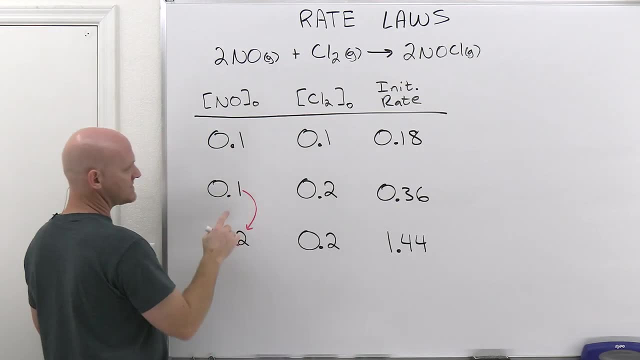 Okay, And trial three that is going to help us. The only change is the change in the NO concentration, And so in this case, as we go from trial two to trial three, we can see that the overall concentration here is going to double. 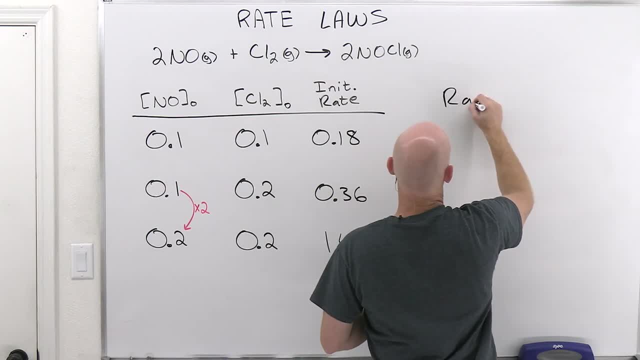 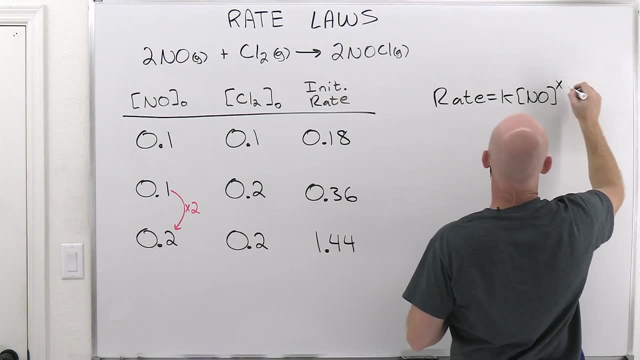 And so if we take a look at what this rate law might look like, here we've got rate equals K, And again we expect our reactions to show up here. So NO, we don't know the order. and then CL2, and again we don't know the order. 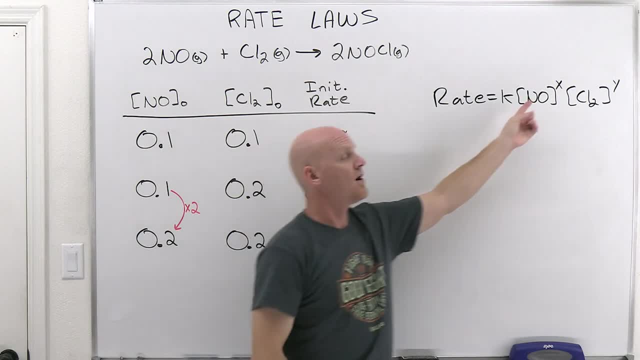 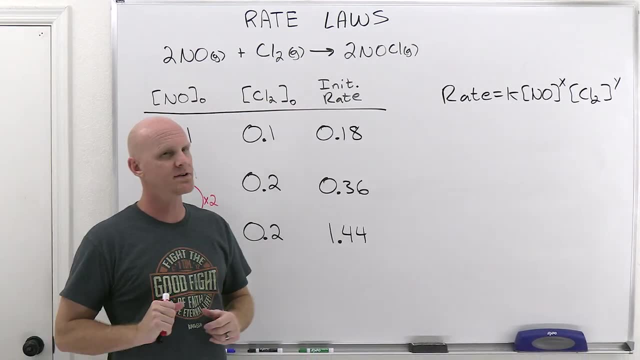 You can't just assume that these coefficients in the balanced reaction are the orders. It sometimes works out that way. It commonly doesn't. There's no way to know, although we'll see one caveat to that in a little while later in this chapter. 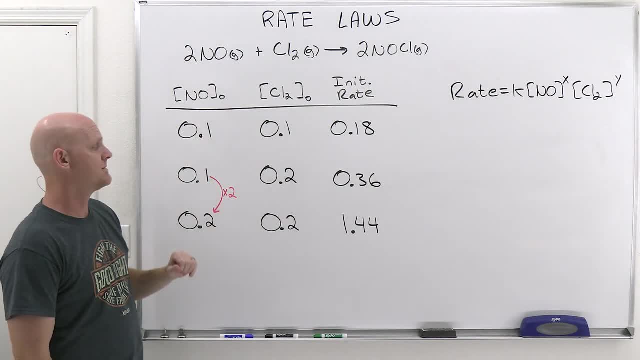 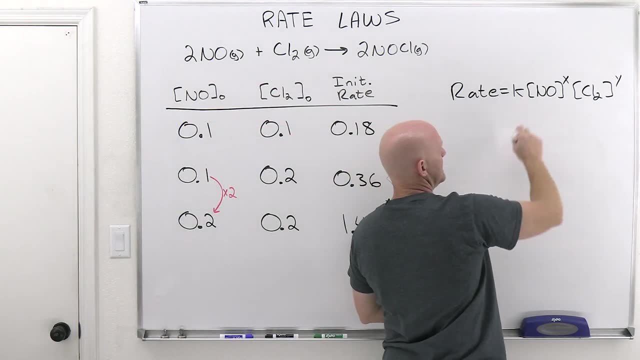 So, but the experimental data is ultimately what's going to tell you. those are, And so in this case, we can see that the overall concentration of NO doubled. And so in this case that NO concentration is doubling Now, the rate constant isn't changing. 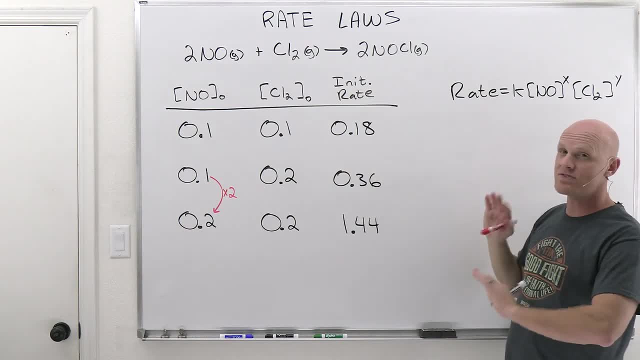 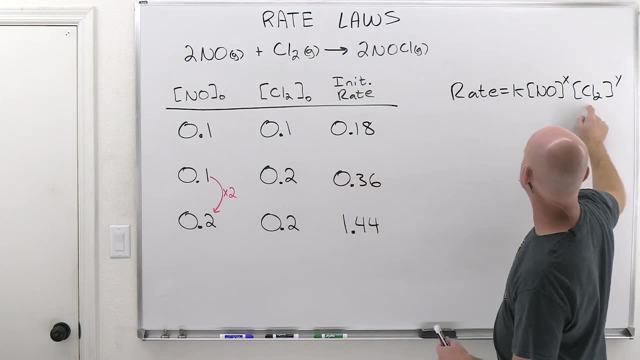 We'll find out that you can change this if you change the temperature or something like that, But it's not changing in this case, in principle. And we didn't change the CL2 concentration going from trial two to trial three, So this is not changing. 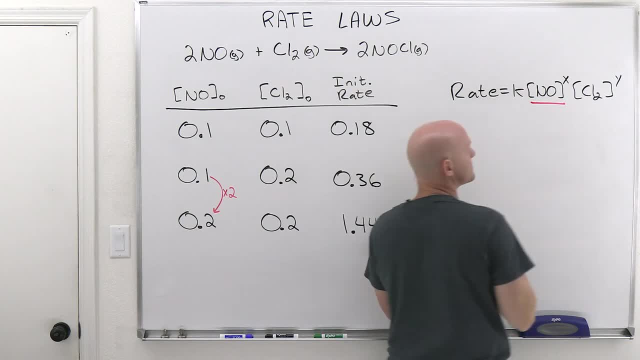 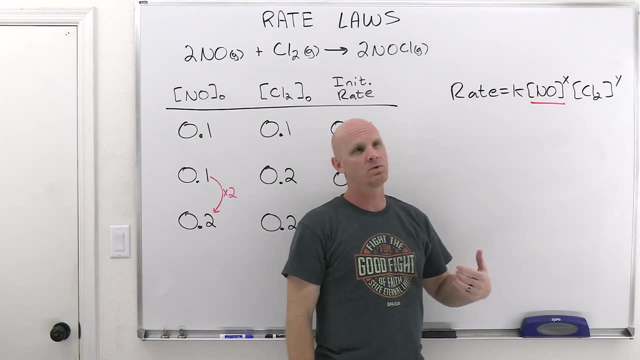 And so the only thing that's changing here is that NO concentration And the rate's going to have a corresponding change to the power. But if that's a zero, well then it's not going to change at all, because anything to zero power is one, and anything times one is itself. 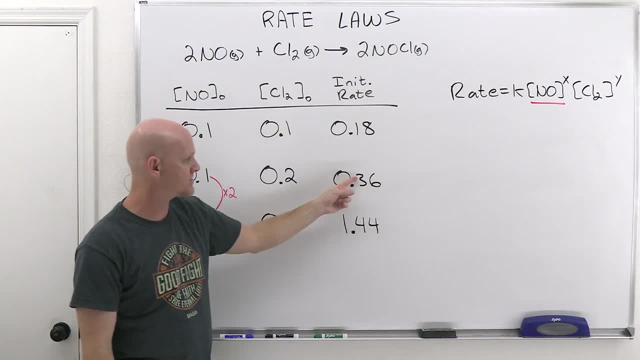 And so if it's zero order, then the rate's not going to change. Well, if we compare trial two to trial three, the rate changed. Okay. Well, then it's not zero order. Now, in this case, if it's first order- and again we're really just going to consider: 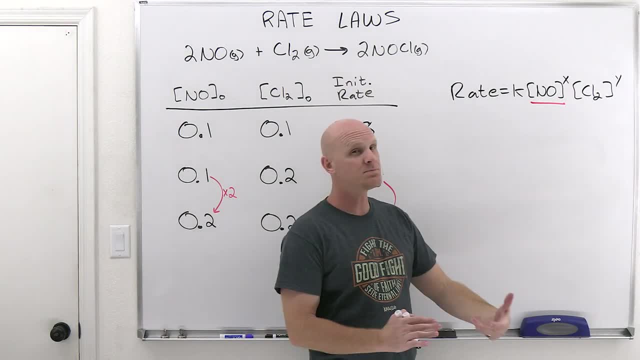 zero one and two the integers. So again, in principle they could be fractions or things of this sort. In that case, like in the lab, we'd have a different way of kind of going about to solve what these orders are. 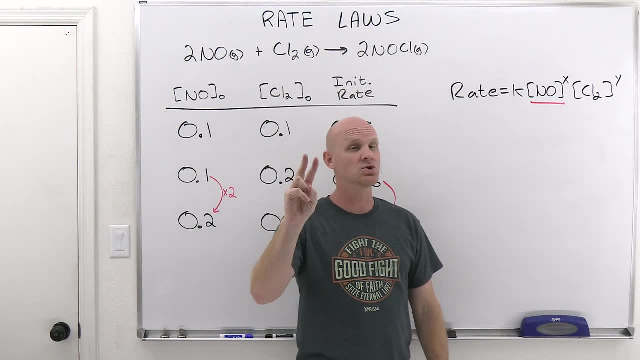 But in this, in kind of in the lecture, it's either zero or it's going to be one, or it's going to be two and maybe three, And we don't have to worry about, you know, some complex stuff involving log calculations. 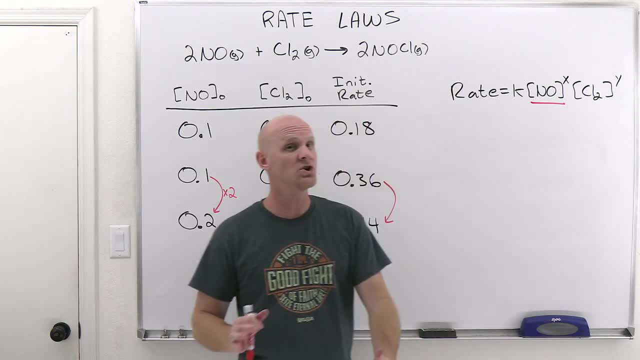 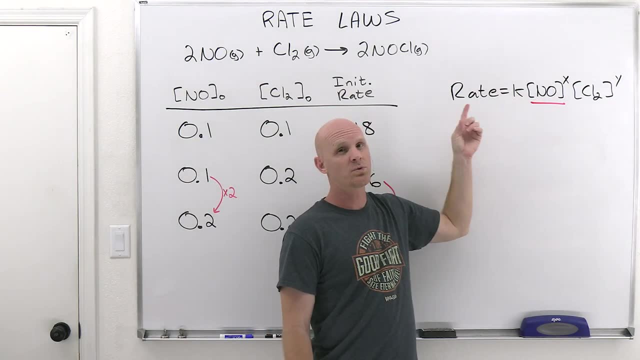 and stuff like this. to figure it out, We're just going to assume it's either zero, one or two. Okay, Either one or two to begin with, or possibly three, And so in this case, if I know that you know the NO concentration doubled well, the rate's. 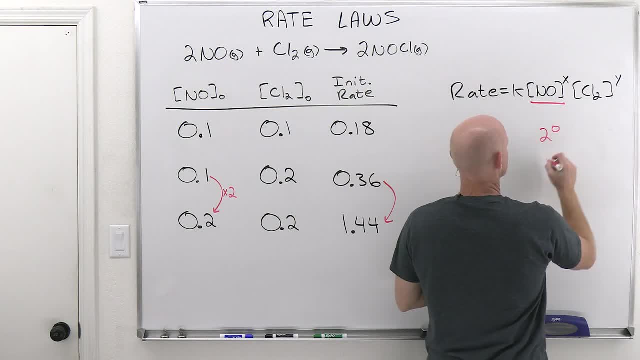 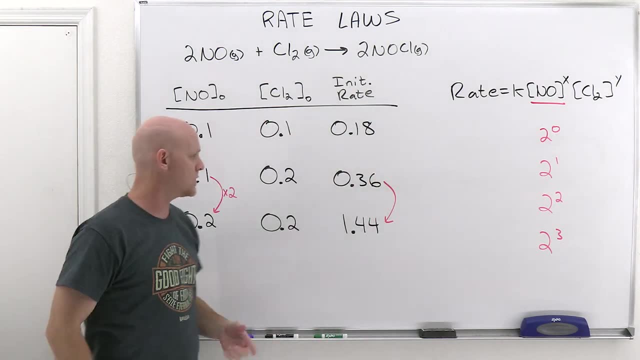 either going to go up by a factor of two to the zero, two to the one, two to the two or, really rare, two to the third power. And the question is really just which one did it do Well, going from 0.36 to 1.44, it turns out 0.36 times four is 1.44. 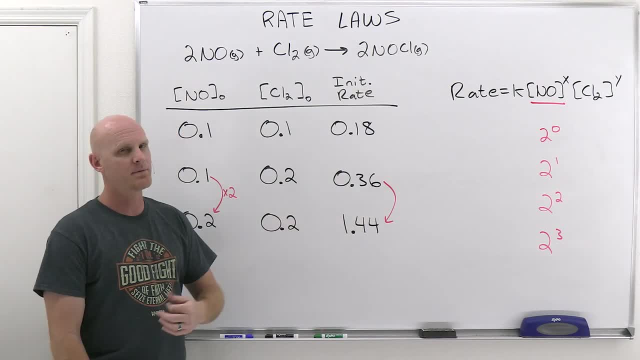 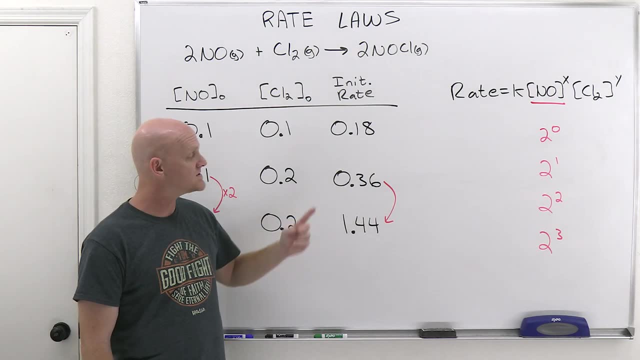 Or, if you want to do: 1.44 divided by 0.36 equals four, probably the better way. This is a fourfold increase, not necessarily the easiest one to see in your head, but notice: 36 times two is 72 and 72 times two is 1.44.. 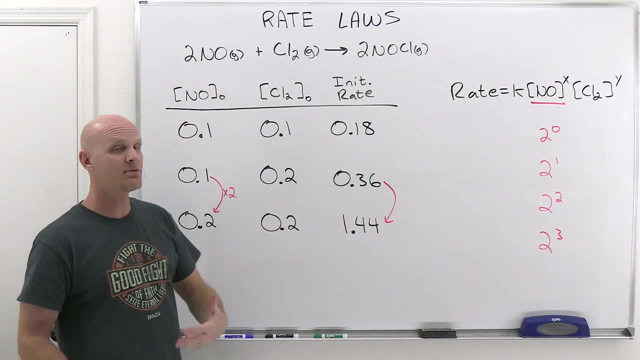 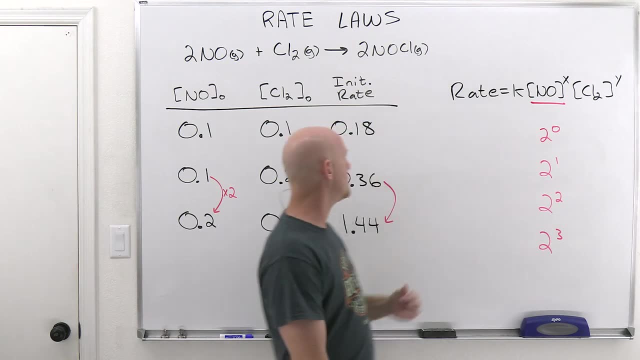 So 36 times four is 1.44.. You want to look at it that way, but definitely use your calculator. but this increased by a factor of four, And so the question is: what exponent lines up with that? So the concentration of NO again doubled, but the rate went up by a factor of four. 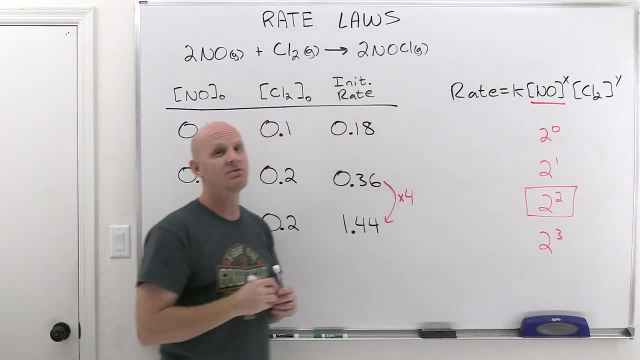 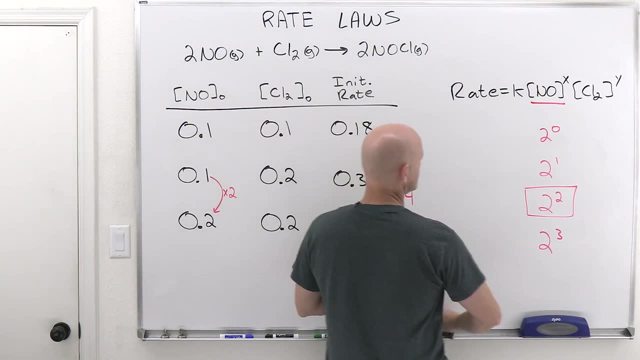 Well, two squared equals four, And that's how we know that it's second order. Okay, Okay. And so the key was: you know you could have gone back and said, okay, well, so what did the concentration do? 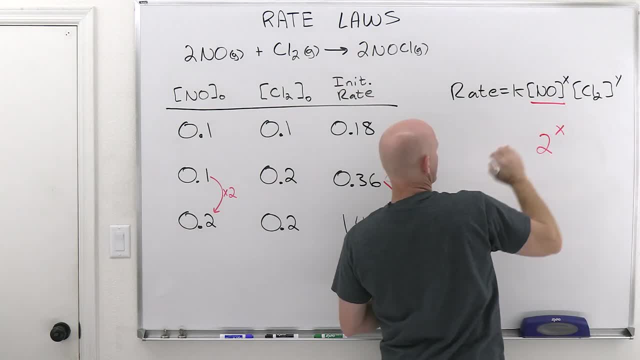 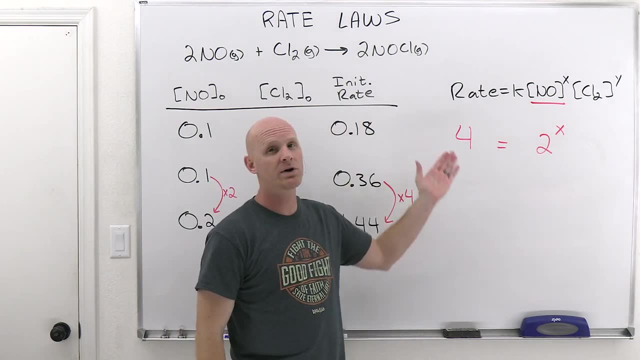 Well, the concentration doubled. So to the X power, according to the rate law. and then what did the rate do? Well, the rate went up by a factor of four. Then what must that exponent be? Two to what power equals four? 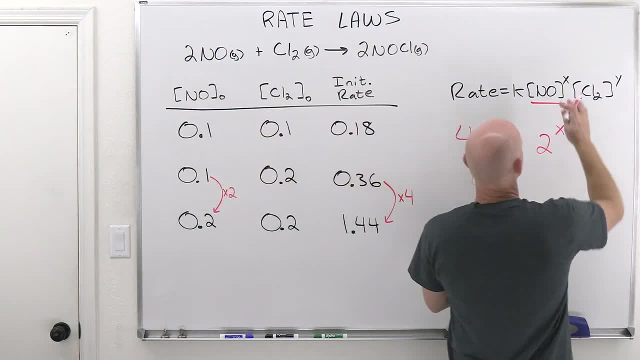 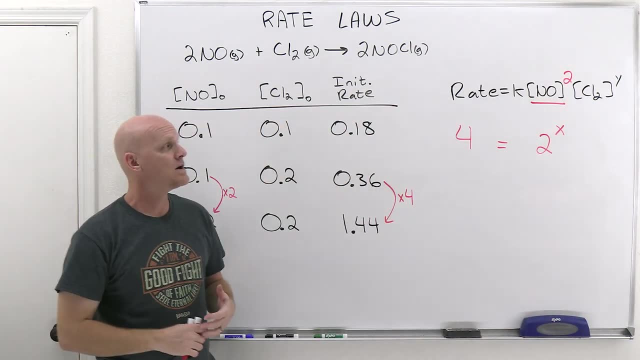 Well, two to the two, power two squared equals four, And now we know that this order right here is a two. Okay, So so far, so good. Now, if we want to find the answer to this question, we're going to have to find the. 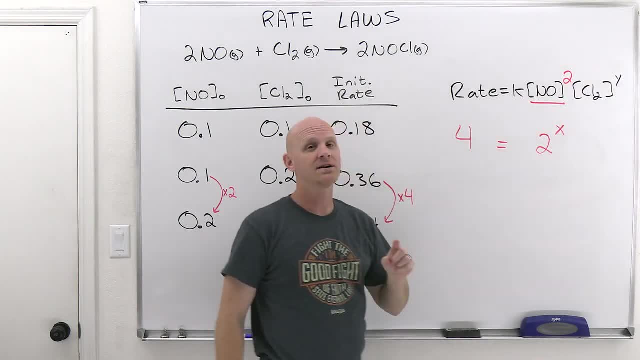 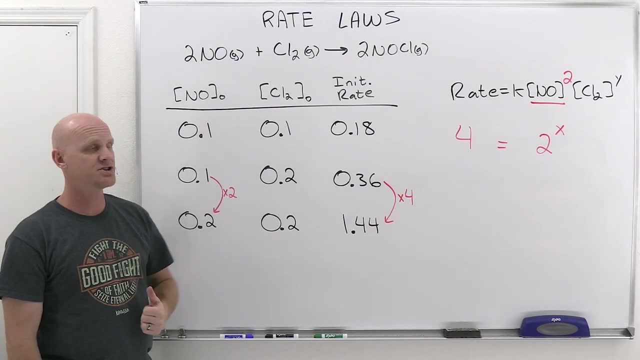 order with respect to CL2.. Again, if we can find two trials where CL2 is the only concentration of either reactant that we change, that we allowed to be changed, then we got a comparison we can make. And so again, notice two to three: that's not going to work. 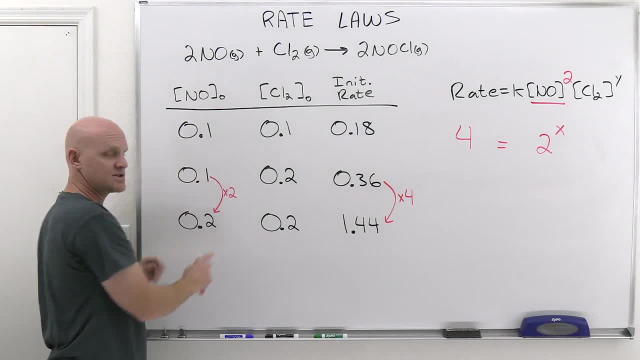 And again we said, comparing trial one to trial three, where they both change, is not really going to be the most helpful. but going from trial one to trial two, So the CL2 concentration once again doubles, So just like the NO did in the comparison we made, and the NO concentration is not changing. 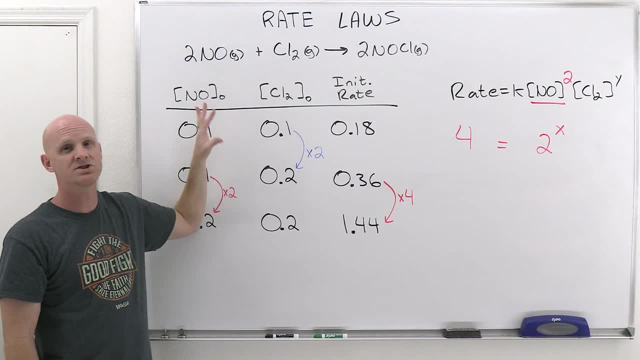 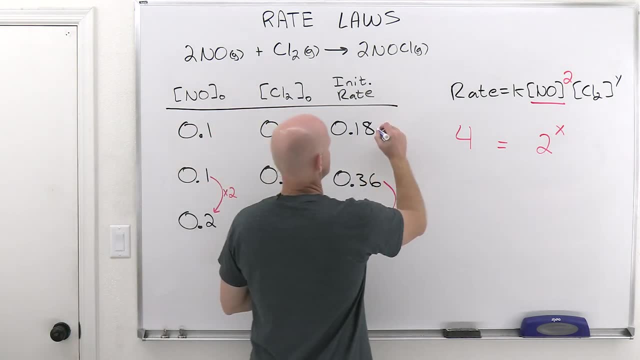 And so in this case, only the concentration of CL2 is differed between these two trials. And so if the rate changes- and it does- I know that CL2 is responsible. And so in this case, if we take a look at going from 0.18 to 0.36, what did that rate? 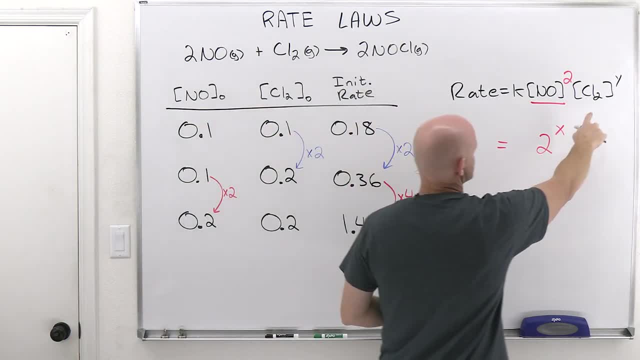 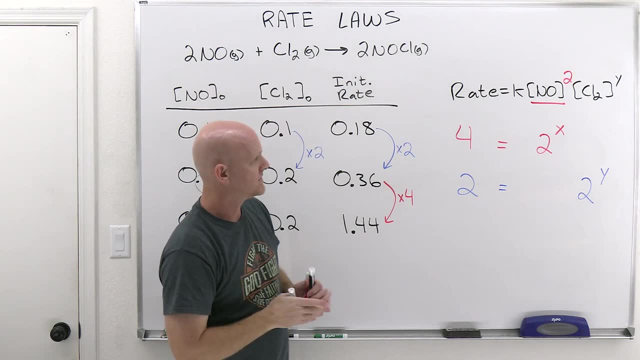 do. Well, it also doubled. And so, in this case, the concentration of CL2 doubled to some power. And what did the rate do? Well, the rate also doubled, Doubled. So the rate doubled, concentration doubled. What order is that consistent with? 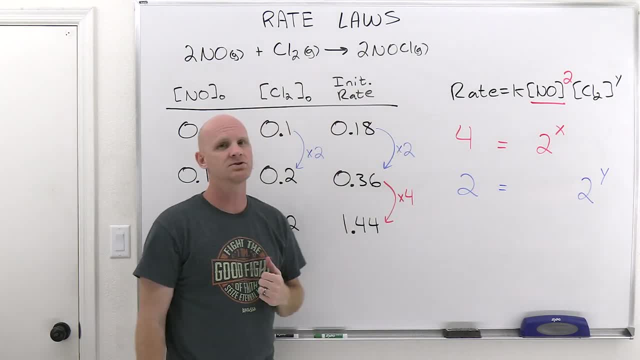 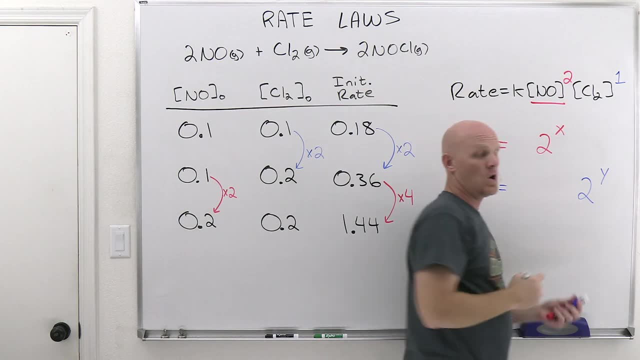 Two equals two. to what power? Well, in this case, that's a one. Two to the one power equals two, And so we just figured out that the order with respect to CL2 is a one, Or, technically, we wouldn't even have to write it in. essentially, 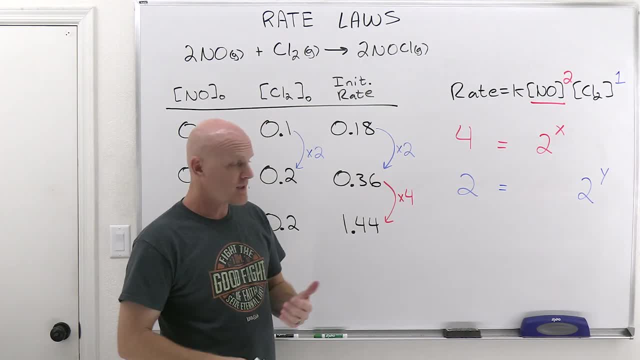 Again, if there's no order written, it's implied that it's a one. So in this case we've now figured out that the order with respect to NO is second order. We figured out the order with respect to CL2 is first. 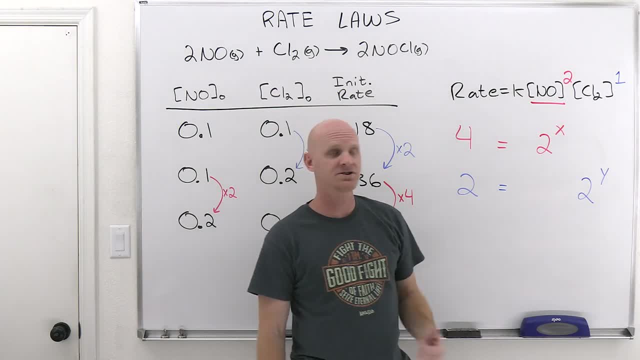 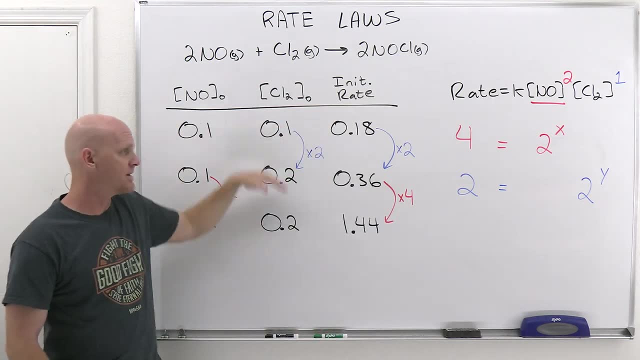 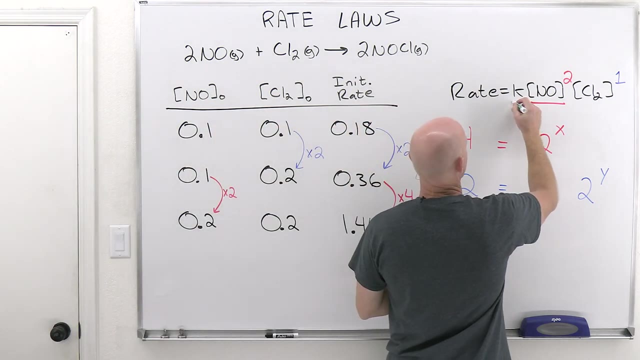 And if I said what's the overall reaction order, It would be a grand total of three. Cool. Now the last question you might get asked here from experimental data, and you'd have to figure out the orders first. but the last question could be: what is the value of the? 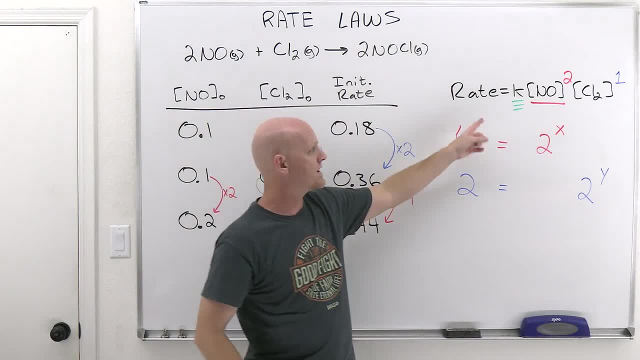 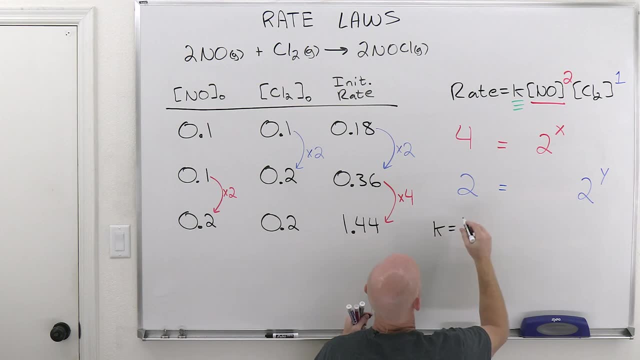 rate constant. And so now that we figured out the orders, we can rearrange this expression to solve for K. And so if we do that here, we've got K equals CL2.. We've got CL2.. We've got CL2.. 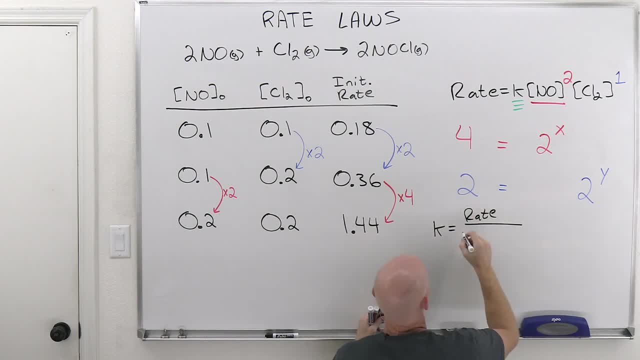 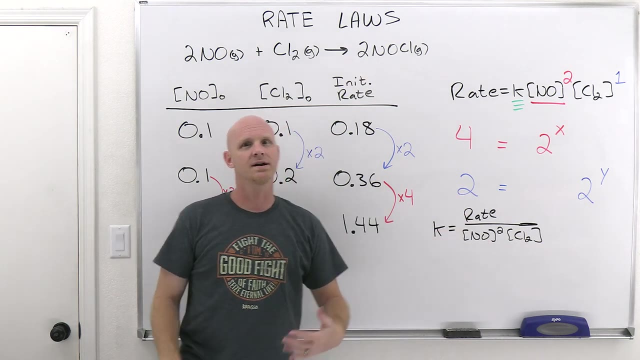 We've got the rate all over. concentration of NO squared times concentration of CL2.. That's the expression for the rate constant. So to be able to figure out the rate constant, I need a situation where I know the rate and both concentrations Well great. 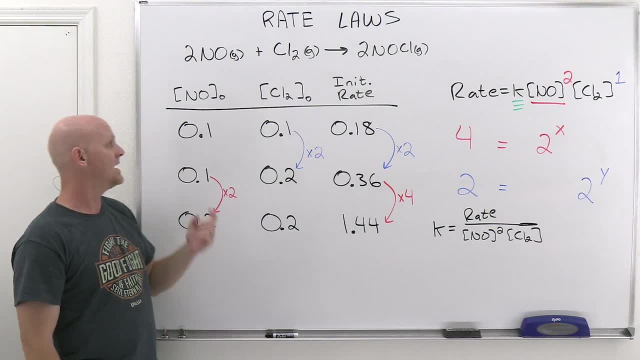 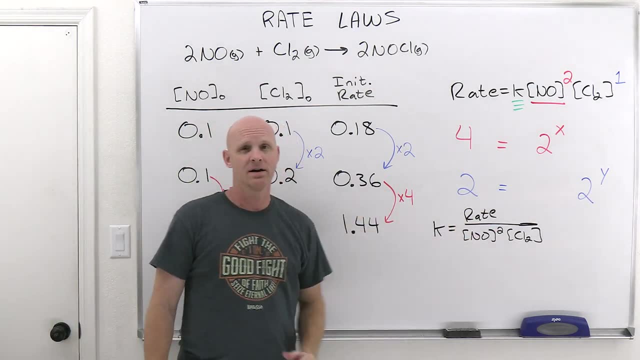 I actually have three different situations where I know all three of those, I know the rate and I know the concentrations of the reactants And I can just pick any one of these trials and plug them in. Now again, if you did this in the lab, you'd know that the concentration of the reactants 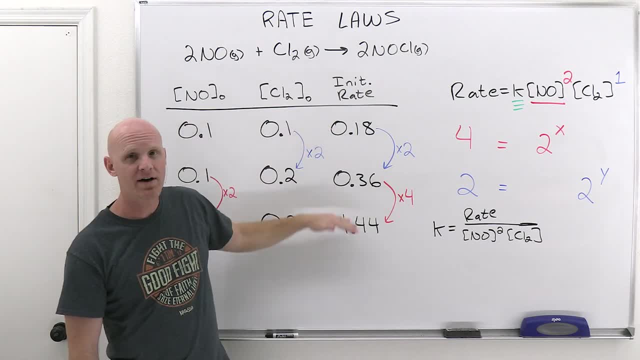 is the same, And if you did this in the lab you might not get exactly the same K value trial to trial, But they should come out close. It is a constant as long as we're not varying the temperature here. But here when I make up the data and I make the data fit the equation, no matter which. 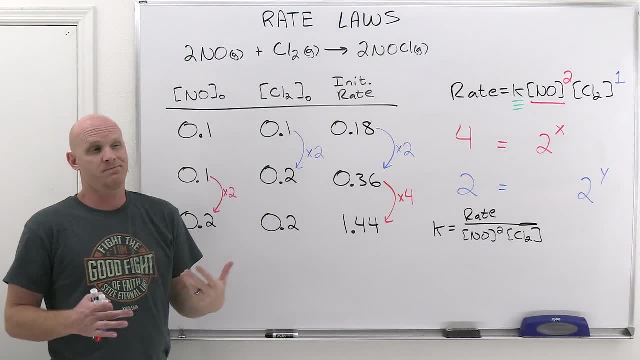 trial you use here, the K value is going to come out exactly the same, And so in your case I would pick whichever trial has the easiest numbers to work with, And I'm just going to use the first one. I like point ones. 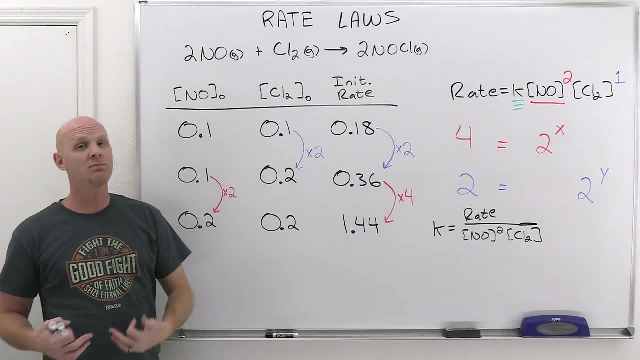 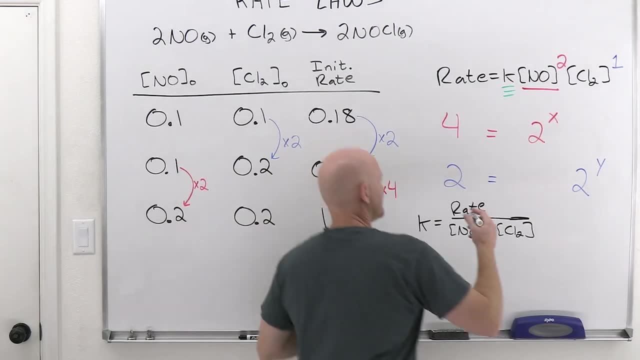 You know, multiplying by point one is dividing by 10, or dividing by point one is multiplying by 10.. And it just makes the math easy without easy access to a calculator for me here. But you should be using a calculator, All right. 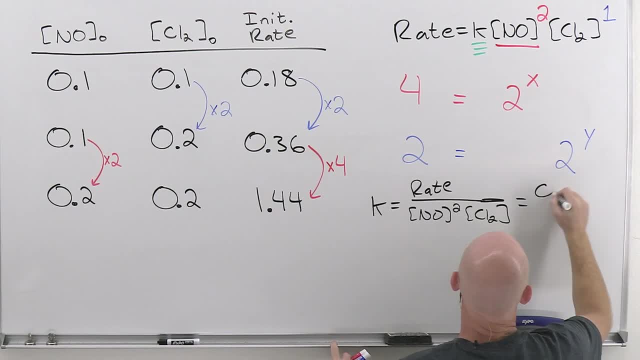 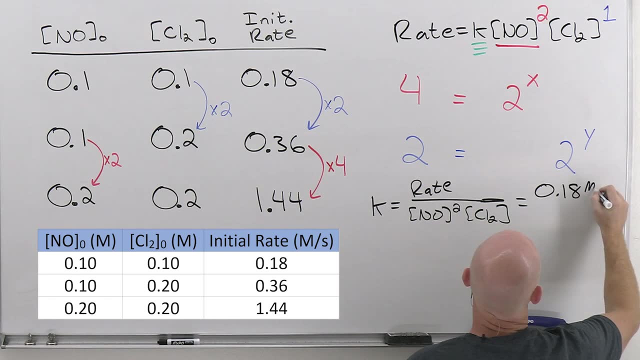 So in this case the rate is 0.18 in that first trial And I'm going to put the units on. I didn't put units here, But on the study guide it's molarity per second for the rates and then the concentrations. 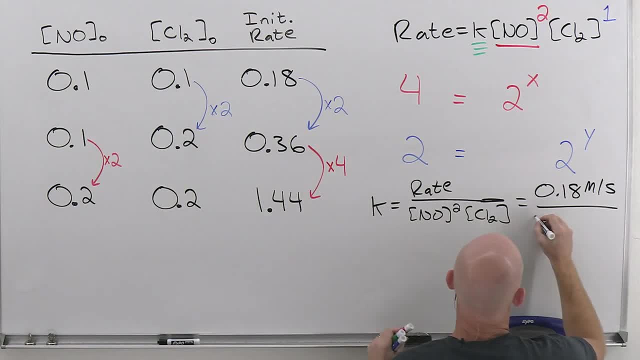 are all molarity, And so the NO concentration is 0.1 molar. So then the Cl2 concentration is also 0.1 molar, And I'm going to almost make a mistake here and forget to square this Cool. 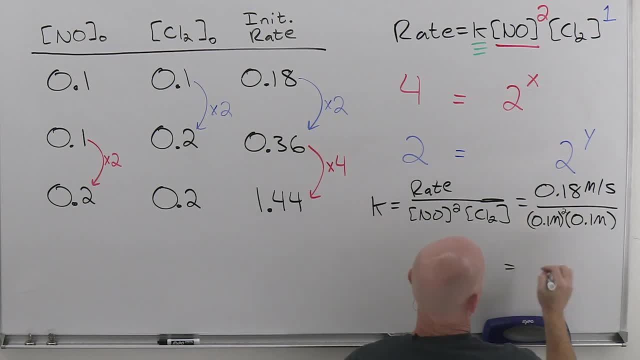 And we're just going to keep track of the units here, And so, if you look, we're dividing by 0.1 squared, which is the same thing as dividing by 0.01, which is the same thing as multiplying by 100.. 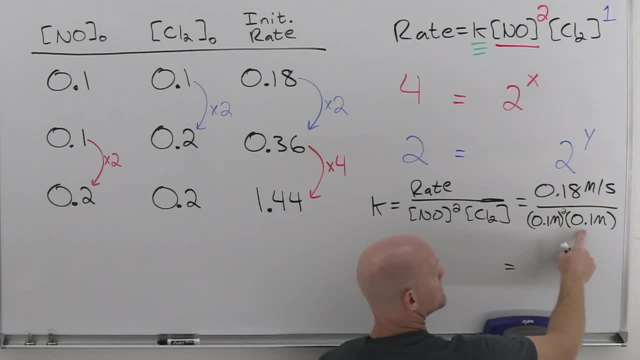 And multiplying by 100, we get this to 18.. Dividing by another 0.1, we'll be multiplying by another 10, gets us to 180.. And if you look at how the units work out, one of these molarities is going to cancel. 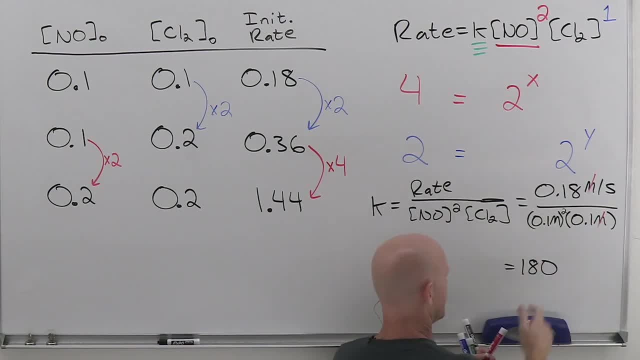 but the other two aren't, And so we've got a molarity squared on the bottom And 1 over. molarity squared is more commonly in these kind of cases going to be written as m to the minus 2.. And then a per second is the same thing as seconds to the minus 1.. 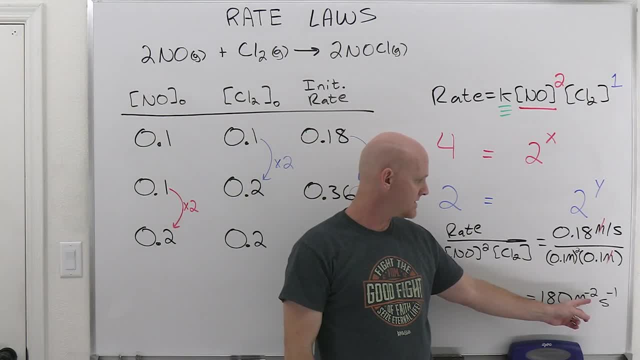 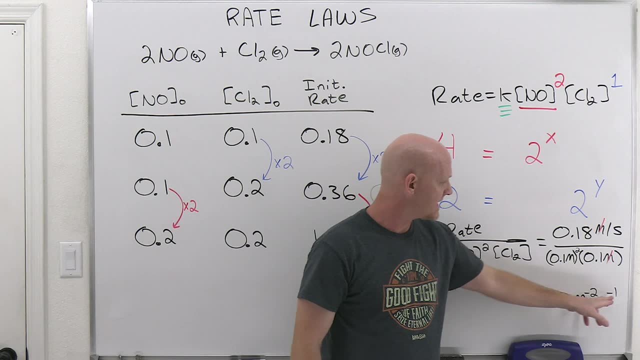 And so what you'll find out if you take the absolute value of adding up the exponent for molarity in seconds or molarity in time, whatever time it is, it's commonly seconds. If you add those together and take the absolute value, it actually is just going to correspond. 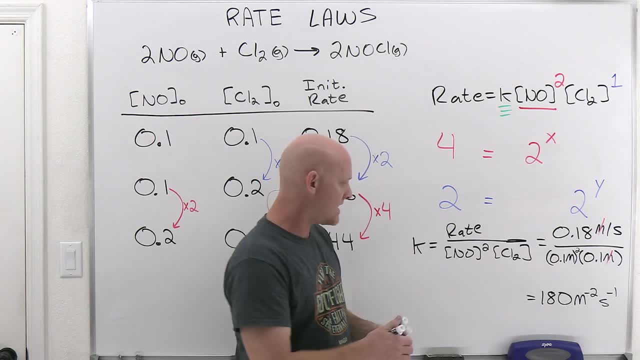 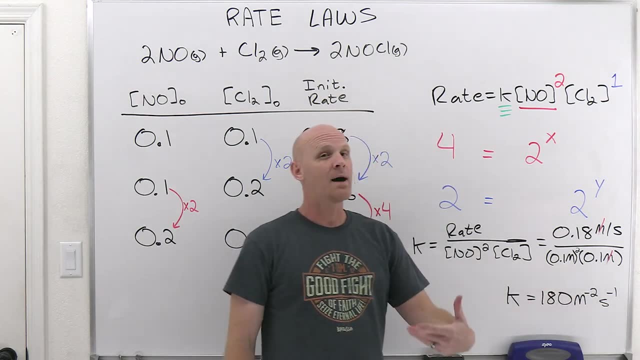 to the overall order, it turns out. So it turns out. the units on these rate constants can be different depending on the overall order of the reaction. So, however, again, negative 2 and negative 1 is negative 3, and the absolute value of 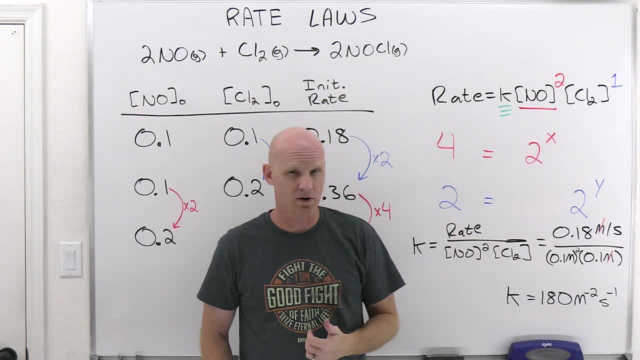 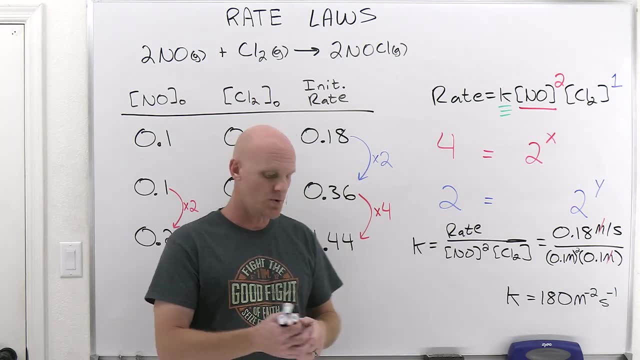 that is, 3.. And this just happened to correspond to third order overall. So there is a kind of a way, if you see the units on your rate constant, of knowing the overall reaction order, And so you kind of see the way this works. 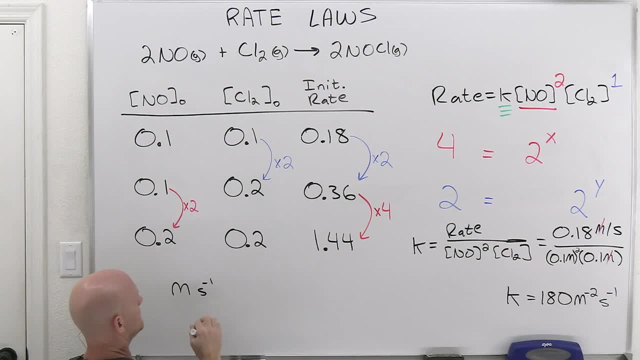 If you have molarity seconds to the minus 1,, well, molarity without any kind of exponent, it's just molarity to the 1, that would correspond to zero order. If I just had seconds to the minus 1, you're always going to have time like a per second. 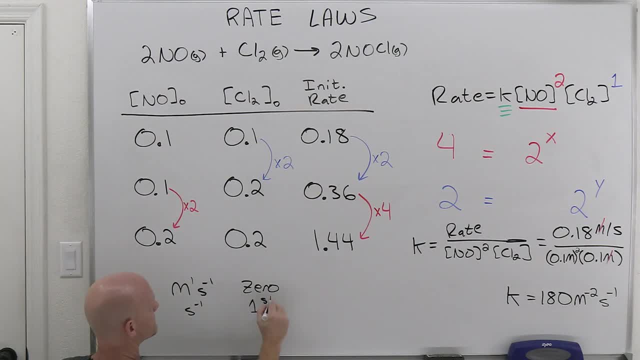 or a per minute, you're always going to have time to the minus 1 power And that would correspond to first order. And if I had m to the minus 1, s to the minus 1, that's going to correspond to second order. 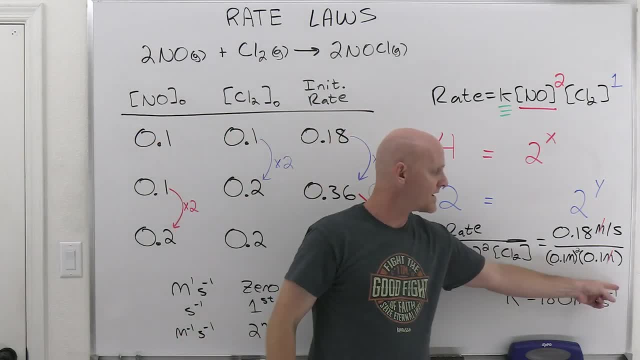 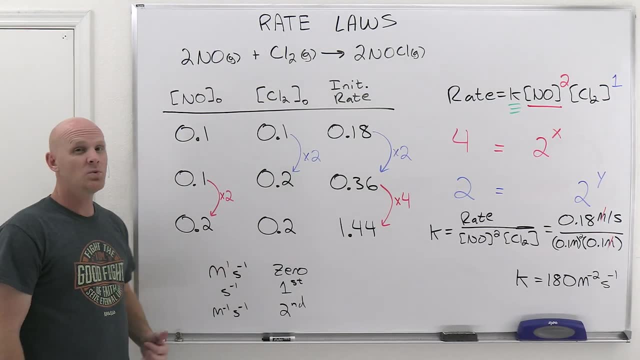 Or, as in the case here, we had m to the minus 2,, s to the minus 1,, and that corresponds to an overall reaction order of third order, And so the units on your rate constant can tell you what order, What's the overall order of a reaction as well. 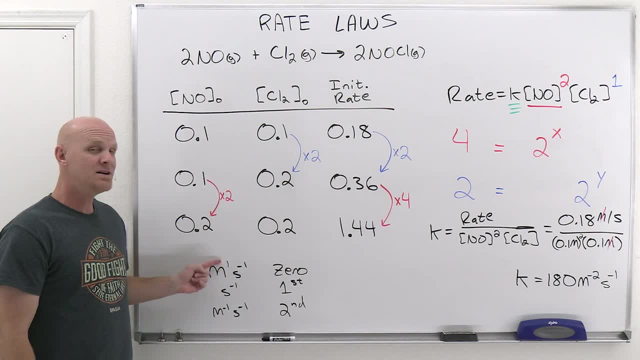 And so sometimes you're going to have to calculate a k value, and sometimes they're mean enough to give you just a difference in units. So, and either you can keep track of your units when you're doing the math, or you can realize. 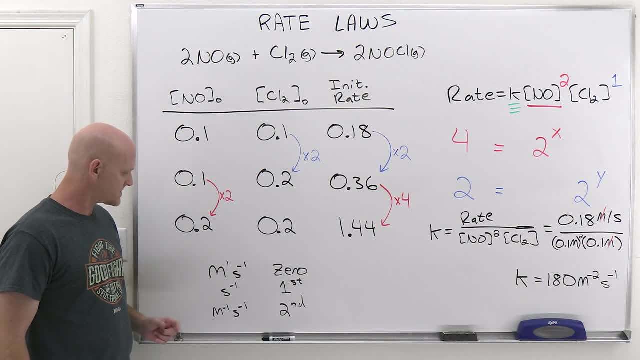 well, if I look at my units, this corresponds to zero order, this corresponds to first order, this corresponds to second order. So if you know your order, you can pick the right units. Or sometimes they'll give you a rate constant and you can look at the units and they're. 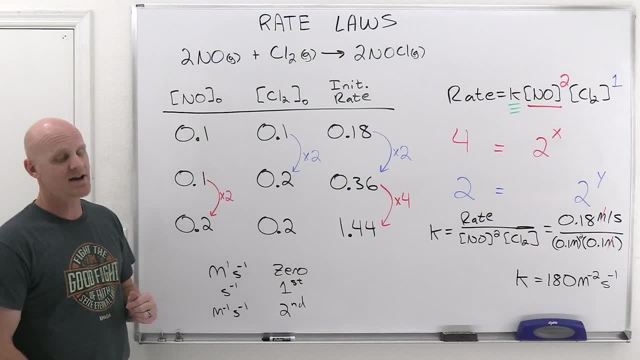 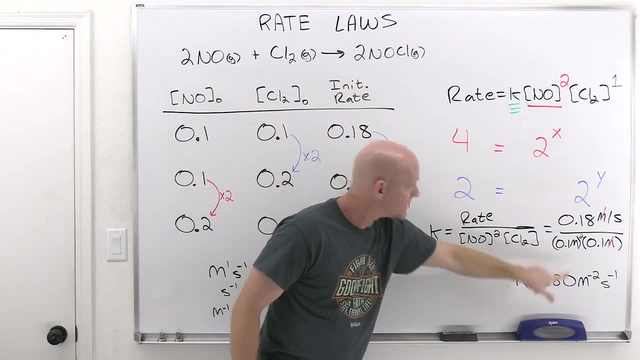 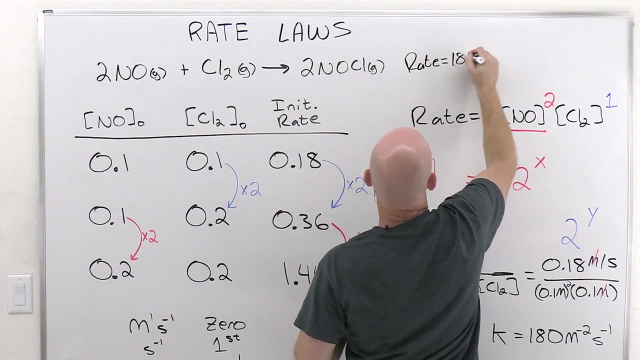 expecting you, based on the units, to know what order it is as well Cool. So one last time here we're going to write this overall rate law now, now knowing the value of the rate, constant, And so if we take a look here, we're going to get rate equals 180.. 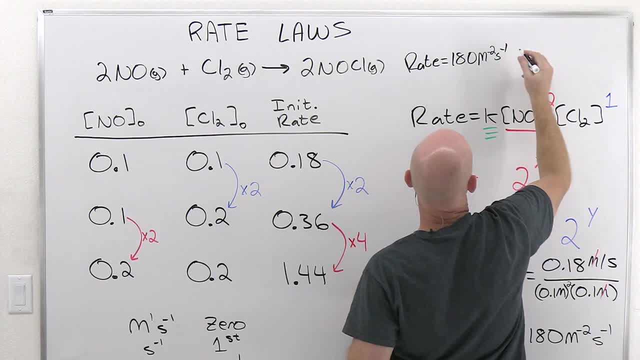 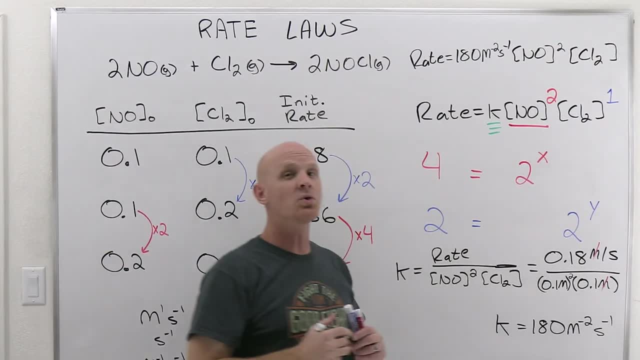 We'll put the units on there as well. So molarity to the minus 2, seconds to the minus 1, times the concentration of NO squared times the concentration of Cl2 to the 1 power which is implied again, And that's our rate law. 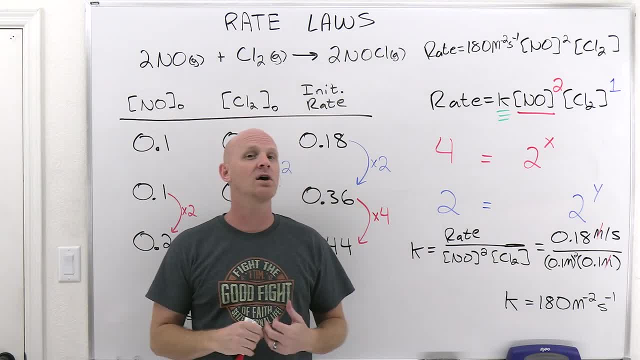 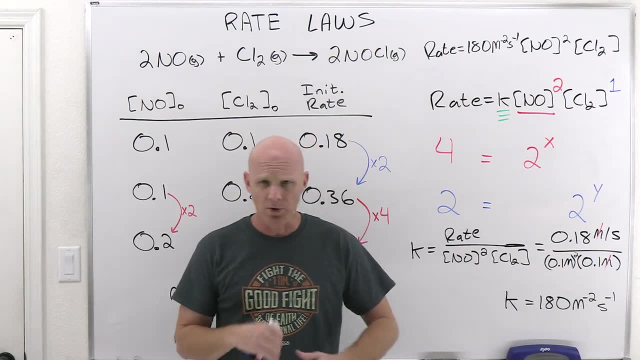 And we said at the beginning of this lesson, The whole point of having a rate law is it allows us to make predictions. And so now, if I said: hey, if you started off with a concentration of NO of 2 molar and a concentration of Cl2 of 3 molar, how fast would the reaction go? 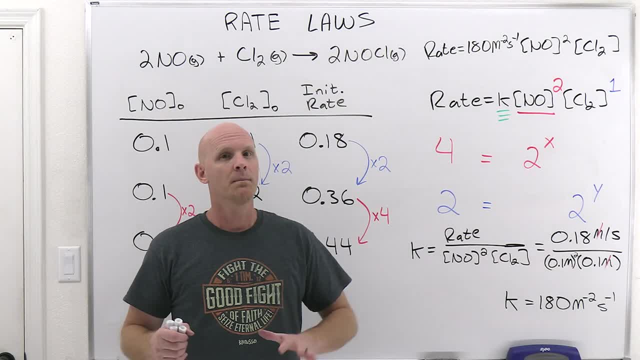 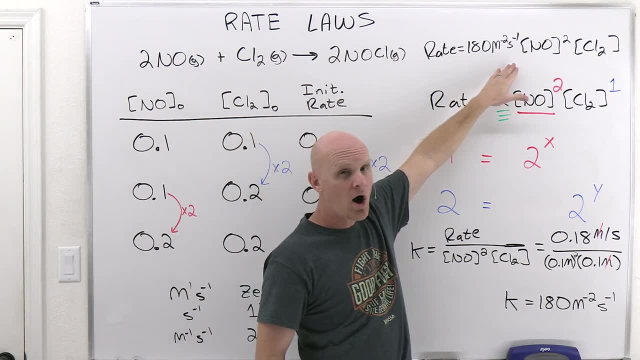 Well, I mean, you could just put those into a beaker and then measure the rate and figure it out. But now that you know the law- just like the law of gravity allows us to make predictions- now that you know the law for this reaction, for the kinetics of it, you don't actually. 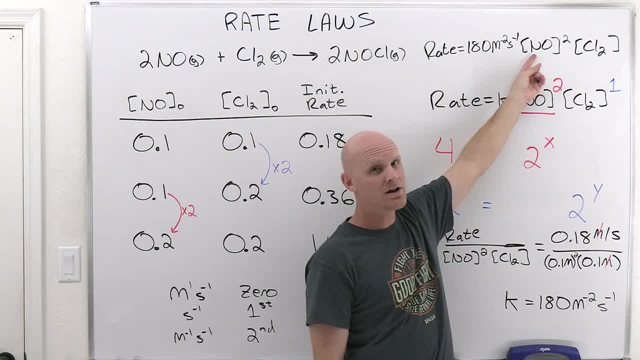 have to run the reaction. You have the law. If I know that, you know the initial concentration of NO is 2 molar, I'm going to run the reaction. If I know that NO is 2 molar and the initial concentration of Cl2 is 3 molar, I can plug.